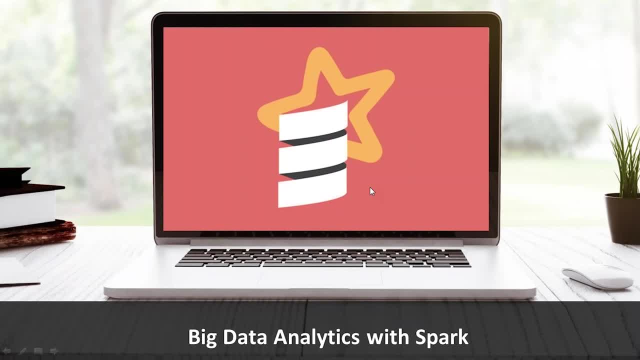 Okay, so that's a quick introduction about myself. I hope my versatile domain experience could help you all in terms of understanding the real world use cases and the big data domain itself, So I would at the moment. I would like to quickly start with the discussion, So apologies for not taking your introductions at this point in time. 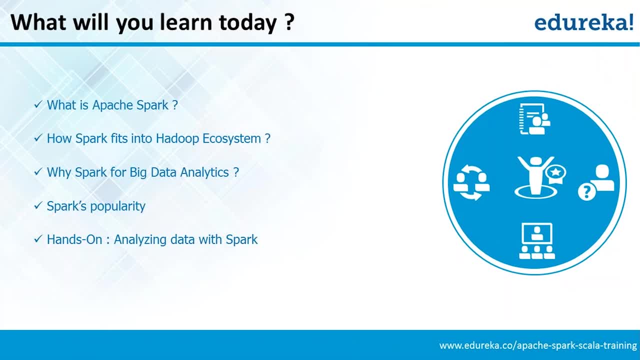 Okay, So in this quick, So in this quick webinar today now, in this one-hour discussion today, what are we going to learn? Let's have a quick look at the agenda for today. First, we will try to understand what is Apache Spark, why there is a need for a new framework when already a prominent framework existing and solving industry problems for big datasets, for example, Hadoop. 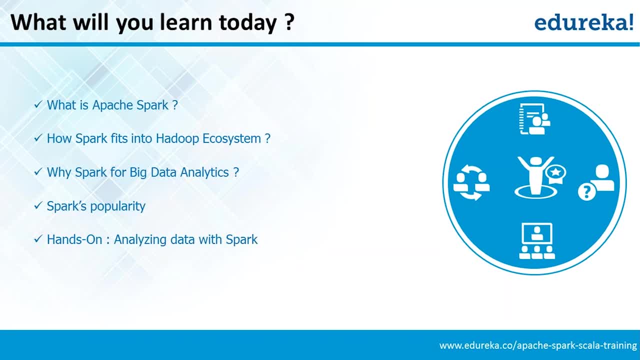 So why? there is another technology called as Apache, Spark, So we'll try to understand that. And then how Spark fits into Hadoop ecosystem. So many of you are a bit confused. I personally interact with many new developers so basically they get confused whether Spark could replace Hadoop or whether it's a complementary software along with the Hadoop. 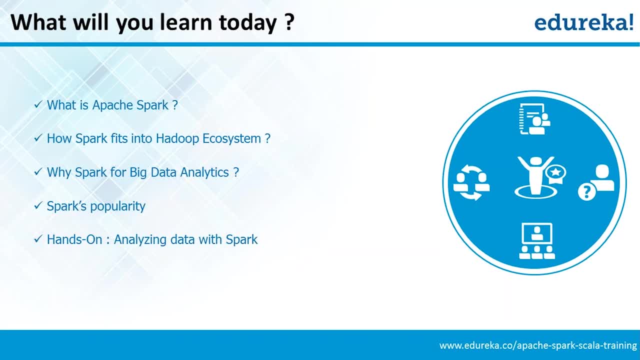 So let's have a quick look at how actually Spark fits into Hadoop ecosystem. Then why Spark for big data analytics? Why, specifically, we need to choose our relay on big data analytics? So here the topic will get more interesting. so that's where I try to explain you theoretically, as well as try to show you certain examples which will help you out in clearly distinguishing the two. 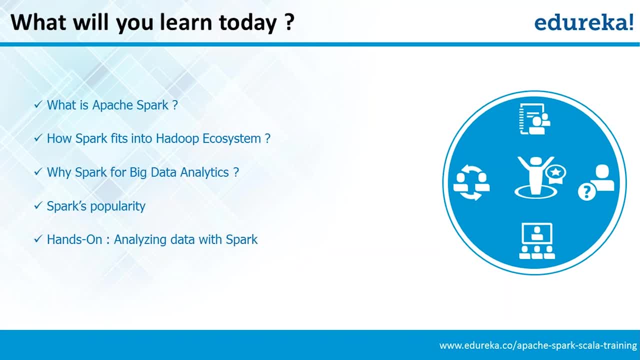 Okay, Let's get started. between the classical way of processing the data on Hadoop versus the Spark, then Spark's popularity. So some of the theoretical slides, which basically gives you an idea on how the Spark future looks like and if you really adopt. 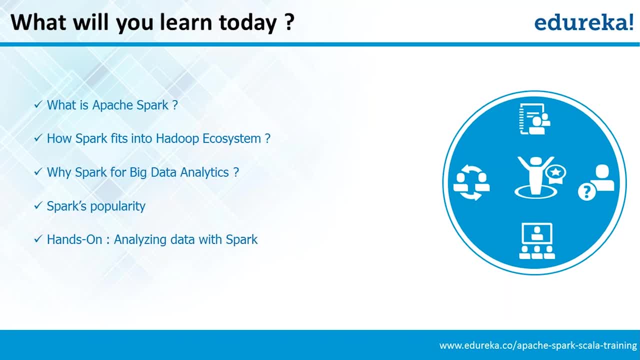 Spark from here onwards. So how would be your carrier part look like? So we'll try to understand that. and finally, we'll try to run a specific complex use case on top of Spark and then we'll try to understand how simple is it it is to implement the code in Spark by solving a really complex use. 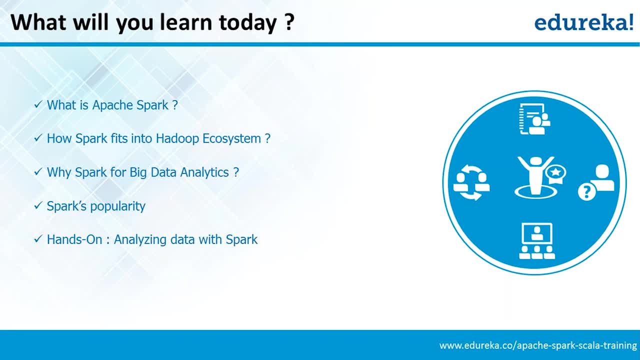 case, we'll probably end our discussion at that point in time, So does that sounds like a good plan for one hour discussion? folks Just say certain, or even Smiley should work Excellent, okay, So I'm sure you guys are quite enthusiastic to go and start discussion. Okay, so let's see. 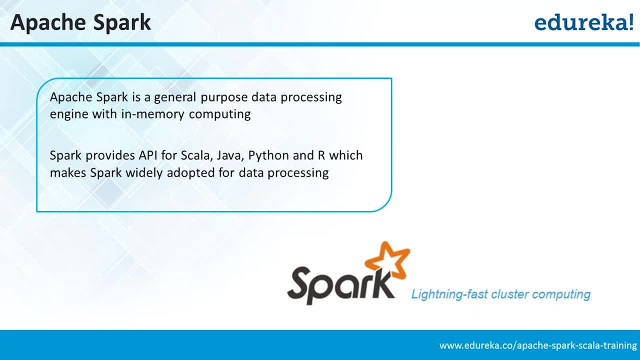 So here is the quick introduction about the Spark framework. So it's basically talks about a. it's a simple definition about the Apache Spark. By the way, it says that Apache Spark is a general-purpose data processing engine with in-memory computing. and then Spark provides API for Scala, Java, Python and R, which makes Spark 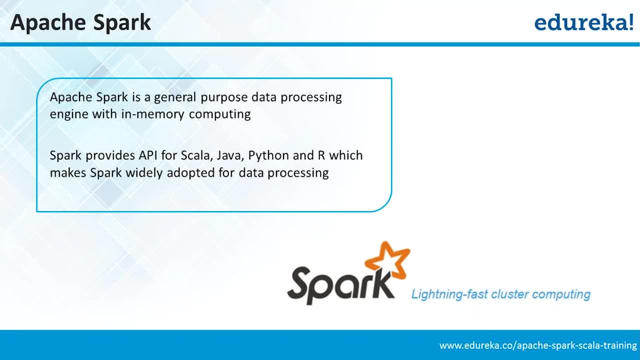 widely adopted for data processing requirements. So let's try to understand each one of these definitions in detail. So, to start with, it says that Apache Spark is a general-purpose data processing engine with in-memory computing capability. So what does it mean? Why am I referring to referring Spark as a general-purpose? 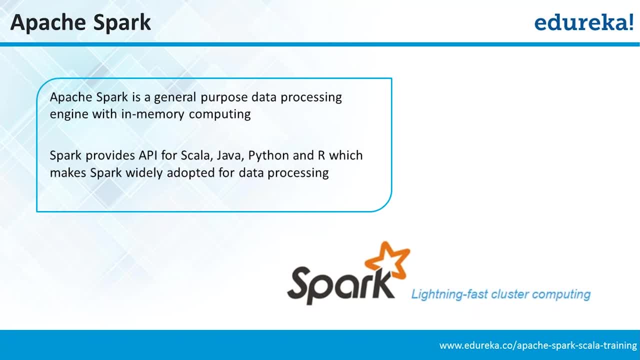 data processing engine. So why am I calling it as an engine in the first place? So let's discuss a few points about that. So, folks, Spark is one of the very interesting frameworks available today in the big data ecosystem which could work as a pluggable engine for multiple underlying data sources. 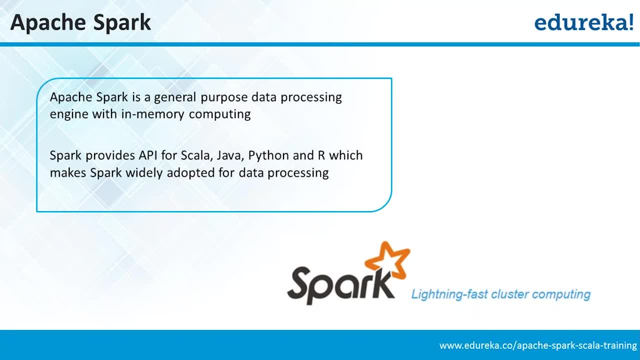 You can plug and place Park quite quickly with most of the underlying data sources available today. For example, one of the most prominent big data source is basically HDFS Hadoop Distributed File System, So you could easily integrate Spark with Hadoop and then quickly run your applications on. 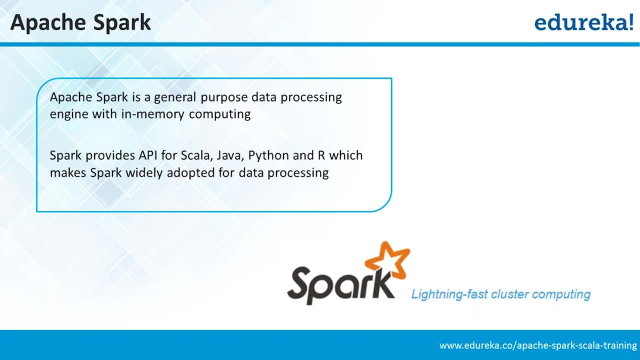 top of Spark rather than depending on top Or depending on Hadoop's MapReduce directly And, as I mentioned, it supports multiple data sources. You could plug and play with additional data sources, for example, NoSQL databases like MongoDB or even Cassandra or many more NoSQL databases available today. 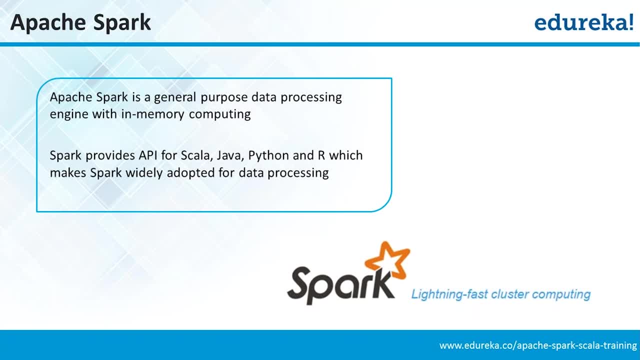 And it's not limited to NoSQL databases, of course. you can even connect it with relational databases, For example, like MySQL, and you can analyze the data quite quickly, compared to that of the primitive engines available to process the data in those data sources. 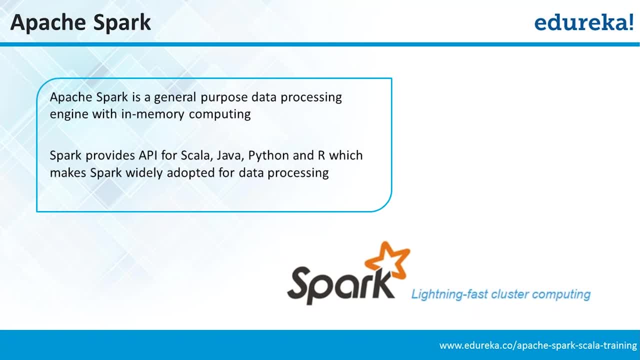 So we will try to understand why it's very fast. It's because Spark has got the ability to process the data in memory. So that's the beauty of Spark. We'll go into the details. We'll go into more details in a few other slides. 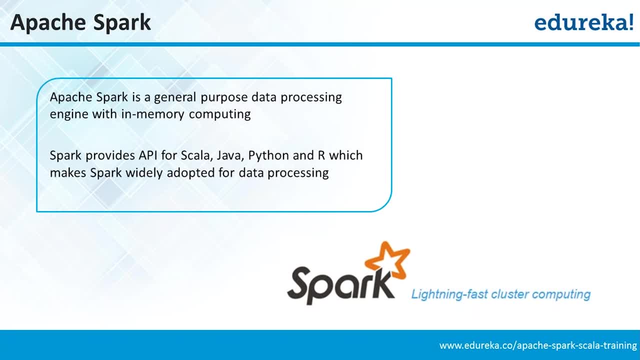 So why I'm calling it as an in-memory computing system, And how does it benefit for an end user or for the developer, at least in our point of view. Okay, So back in 2010,, when I have been extensively working with Hadoop, by then there were discussions. 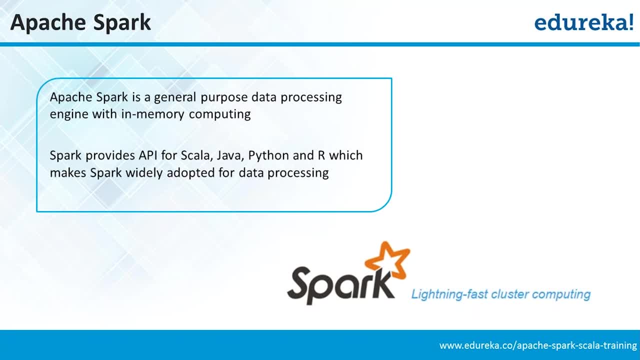 about the in-memory processing frameworks for large datasets, like, say, data residing on top of Hadoop. So if you ask my genuine opinion at that point in time, I had was- I was really confused that whether is it really possible to process such massive datasets sitting on top of Hadoop with. 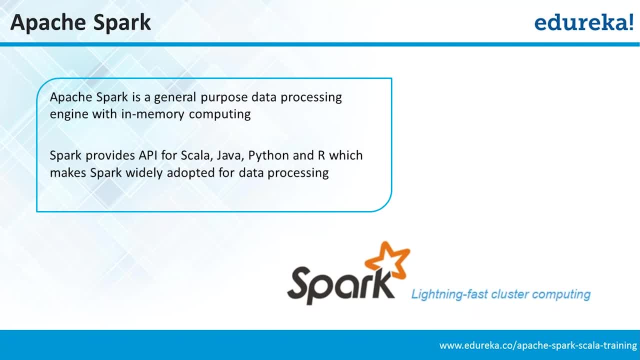 an in-memory processing. Is it really true or is it going to happen, Even though there were a lot of discussions around that in 2010.. Then I started finding out a technology called Spark somewhere in between 2011.. So this framework has got a very interesting internal mechanism with which it could work. 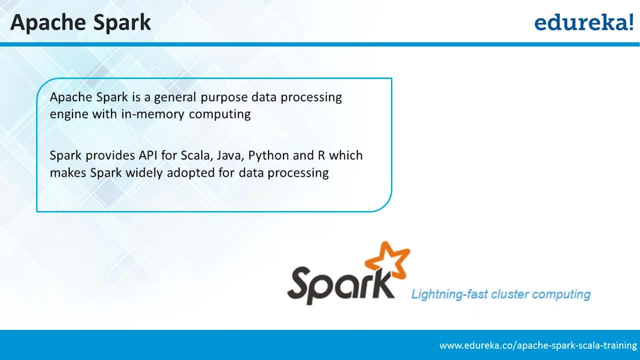 Okay, Spark could be able to load the data across the cluster of machines in memory and then process the data quite efficiently compared to that of the classic MapReduce programming paradigm. Okay, So there are too many technical aspects now, So let's quickly move on and try to understand each one of those definitions in detail. 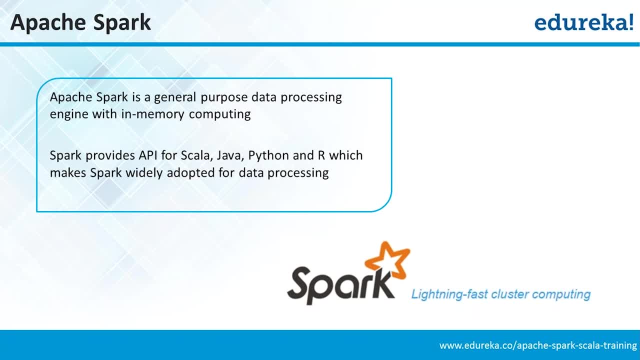 Okay, So before that, Spark provides API for Scala, Java, Python, and even now with the latest releases in Spark, like 1.4, 1.5.. Spark has built very efficient APIs, for example, data frames and some functions with which. 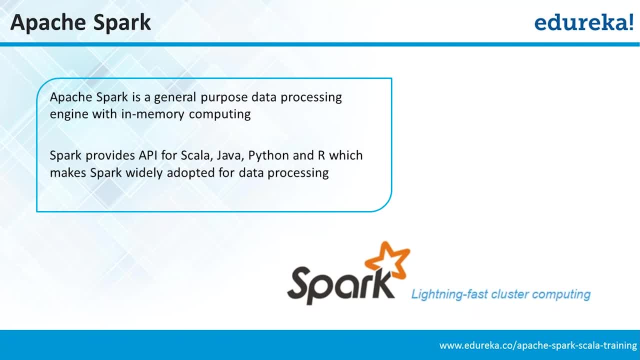 you could be able to easily leverage on the R functions and could run on top of Spark. Okay, So, with the implementation of the data frames and some other functions which are built as part of the R module. So let's move further and try to understand that. 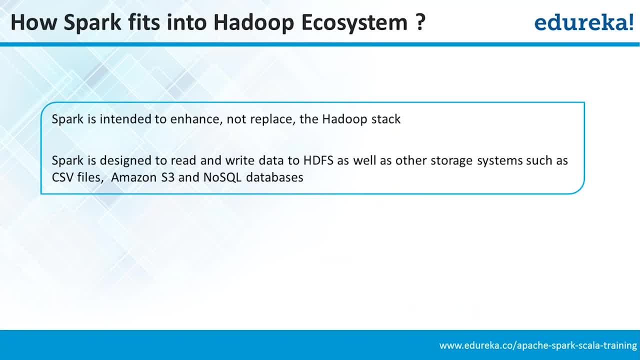 So then, Spark is intended to enhance, not replace, the Hadoop stack. Okay, So, before going further, So there are a few questions, Right, Which I would like to take at this point in time, and then we'll move forward. So Ganesh says: I have, okay. 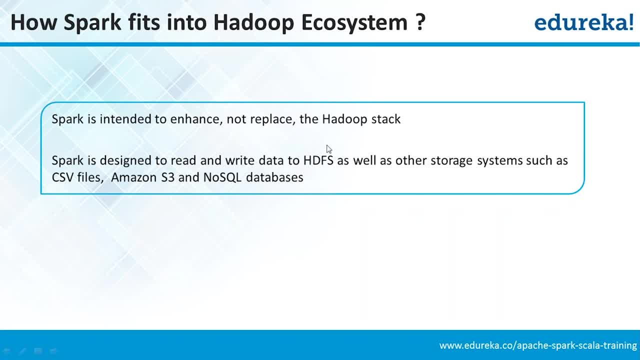 So I think there are some specific questions related to their working, their current situation. So I would like to address such questions at the end of the discussion. Ganesh, sorry. And then Parvik says: actually in memory computing system, Okay. 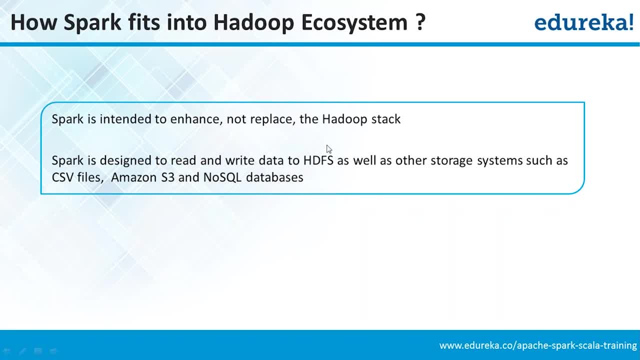 Okay, So I think that we lost the processing data And so we can't validate our algorithm when developing a code. So how could we resolve this? Sure, So I will definitely address this question at the end of the discussion, Parvik. 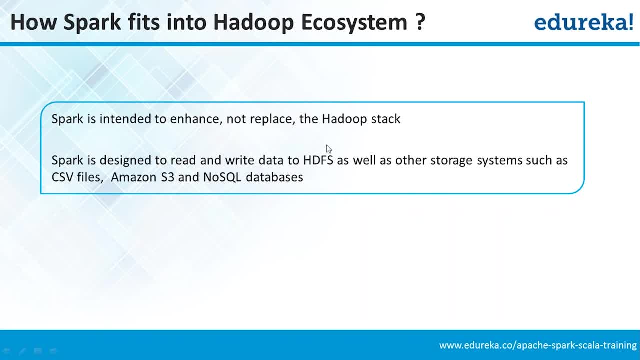 So I'm not going to take questions which are not related to the context, So which could easily disturb the session. But don't worry, I'll definitely help you out in answering those questions at the end of the discussion. Okay, So Vijay says: how does Learning Spark help senior QA professionals? 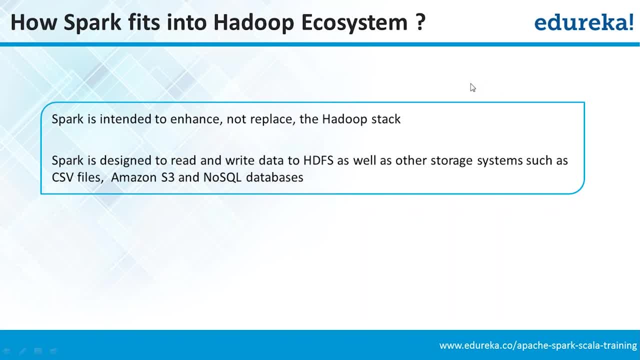 Okay, So I think there are some very, very interesting questions from Parvik and some others, So I will pick up such questions at the end of the discussion. So please bear with me till we finish our discussion, folks. Okay, I'll give you maybe roughly about 15 to 20 minutes time to answer your questions. 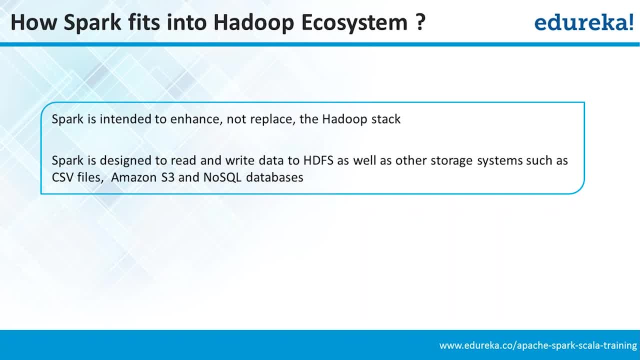 All right, Thank you, Bye, 연습j. married the imperfections okay, since Park is intended to enhance, not replace, the Hadoop stack. Cittous, very, very important and crucial statement to understand for all of you. it's because many of you 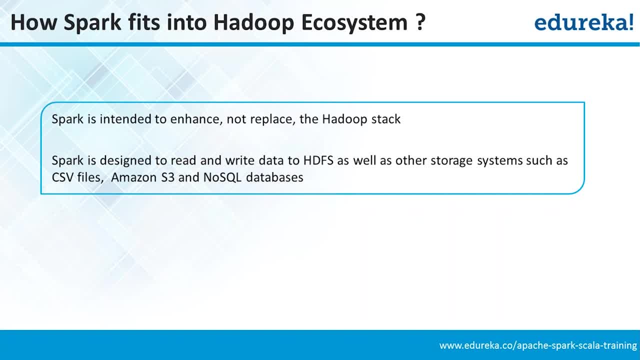 In fact, In the forums I continuously have frequency interact where I see the questions related to of this project can replace sure to, which is totally wrong because help Hadoop nonsense, Its popularity. it's not only because of the MapReduce programming paradigm, it's mainly 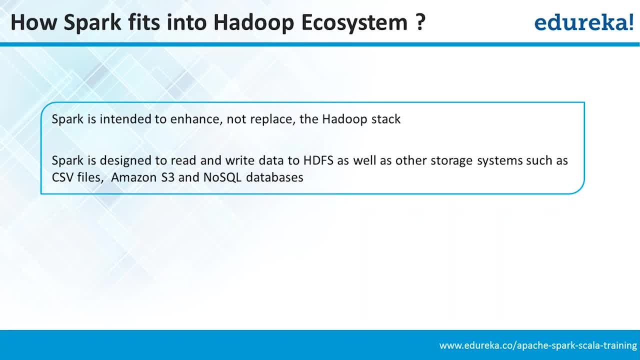 because of its underlying distributed file system, which is the most stable open source technology available with us today, with which you could scale infinitely across any number of nodes over the cluster. with the Hadoop distributed file system And with the advent of Generation 2, a lot of things, a lot of issues have been resolved. 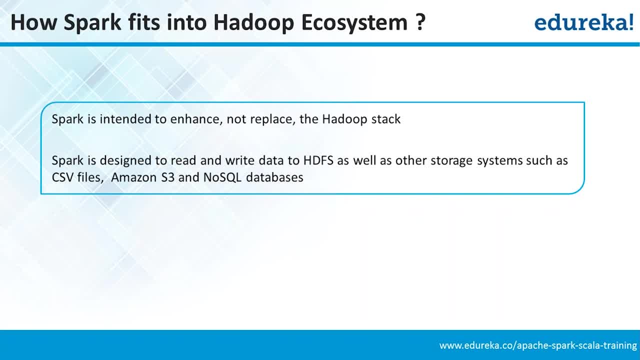 and it has become more stable and more scalable, and many more features have been introduced, like, for example, multi-tenancy. So Spark, on the other hand, does not have its own storage system as of today, So that's very, very important to understand. 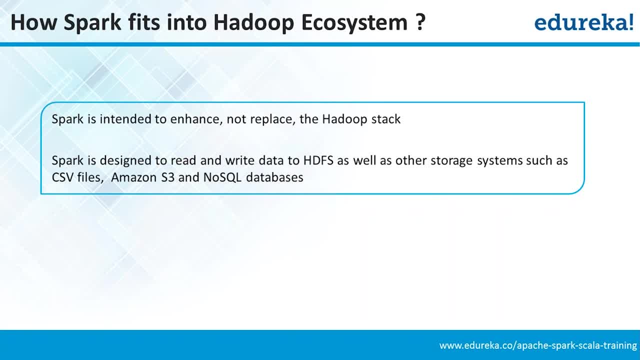 Spark is mainly designed to be a compute engine which could easily be plugged to any underlying data source and can process the data quite quickly and efficiently. So that's the whole idea behind the Spark framework. So then, what is the purpose of actually moving on to Spark, rather than some of the components? 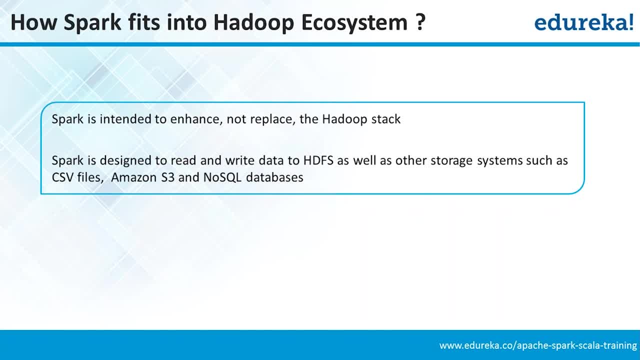 in Hadoop, So let's discuss about that. So, folks, many applications since like last, I would say last- decade have been implemented using Hadoop's MapReduce framework, So it worked very well. It worked very well, It was quite efficient and worked very well for large data sets. 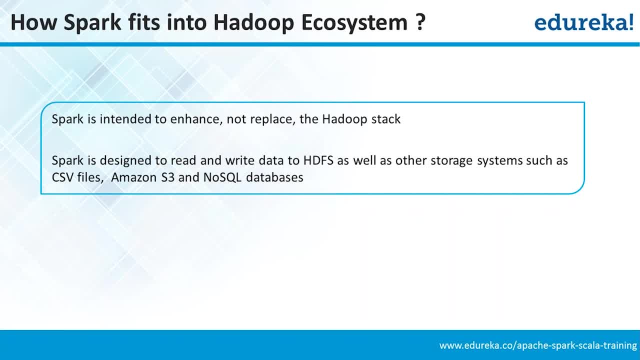 Because Hadoop was initially purely designed for batch processing applications and it fits very well with such kind of environment. But the growing number of communities on top of Hadoop- user communities on top of Hadoop- has started leveraging in Hadoop in different ways. 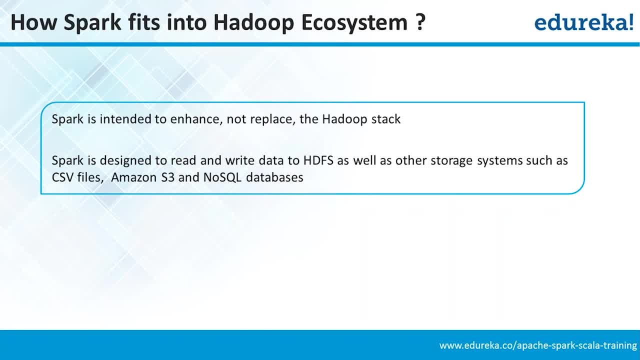 Different aspects. So they started treating Hadoop as a Lambda architecture to process streaming data and then the batch processing data. They started considering Hadoop for real-time applications as well. So that's where the introduction of so many ecosystem technologies has come into picture. 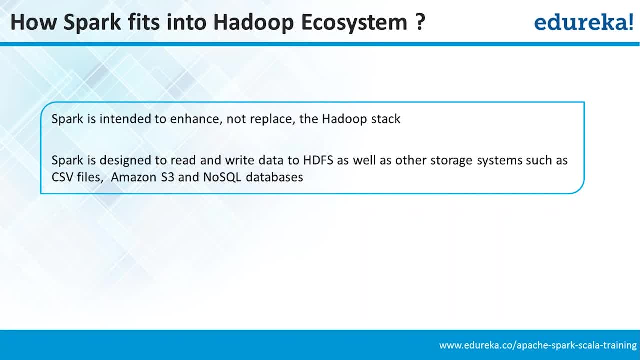 and existence. Okay, So then? Okay. So the Spark MapReduce, on the other hand, is quite high performance computing framework as compared to that of the Hadoop's MapReduce. directly, It's because the underlying implementation is entirely different. the way it does the 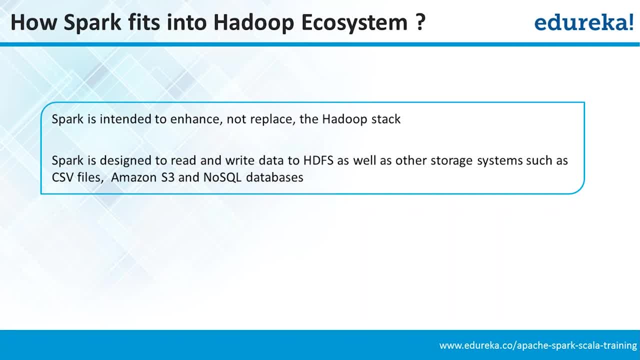 MapReduce. Spark also has got MapReduce Hadoop by default has MapReduce framework. So both the implementations are entirely different. Conceptually both of them are the same Because of the underlying implementation is totally different. you could actually achieve high performance on top of the Spark. 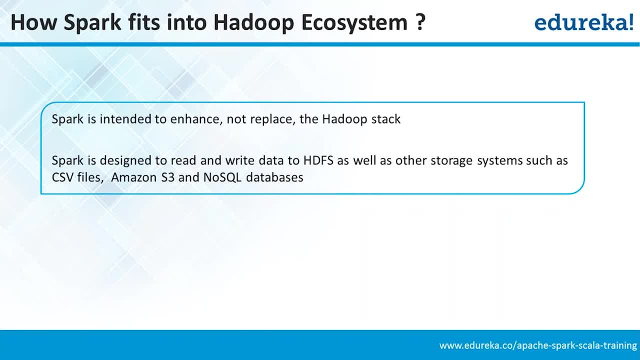 For certain applications, the performance of Spark could go beyond 100 times than that of the Hadoop MapReduce folks. So that's why, even though Spark is not the same as Hadoop, Hadoop is the same as Hadoop. Hadoop is the same as Hadoop. 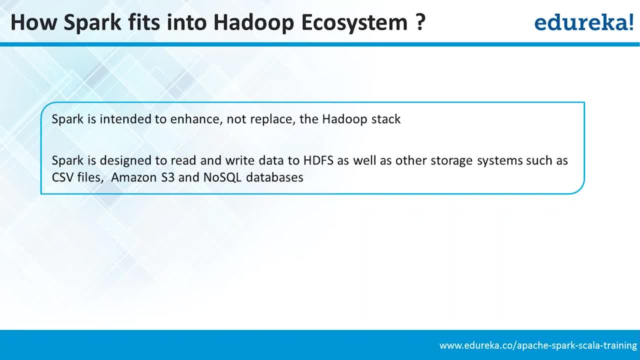 Hadoop is the same as Hadoop Even today. I personally see many of the companies they started totally replacing their existing Hadoop's MapReduce to Spark's MapReduce, Even though there are some conserver related issues which have been solved, which have 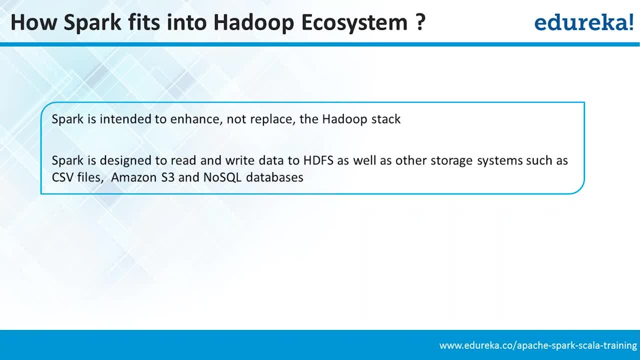 been getting resolved quite quickly because of the number of users, community support provided for Spark, Especialy because of the performance Right Right the Spark MapReduce yields. So Spark is designed to read, So in essence, so Spark MapReduce is quite efficient. 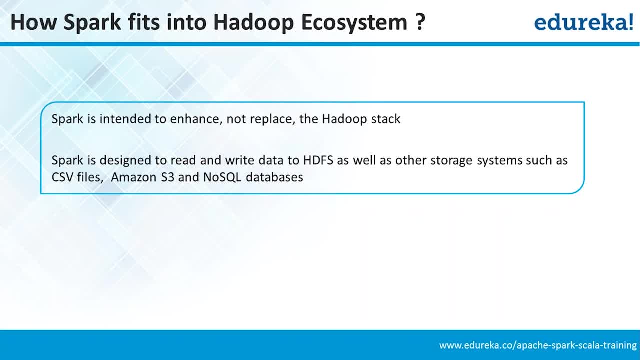 and Spark is not only meant for MapReduce. it has got some another very interesting modules which we'll be discussing in a moment, which also makes Spark more popular and widely adopted framework Are the future framework. So Spark is designed to read and write data to HDFS. 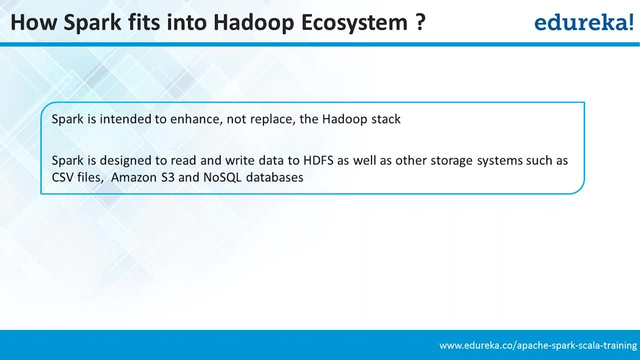 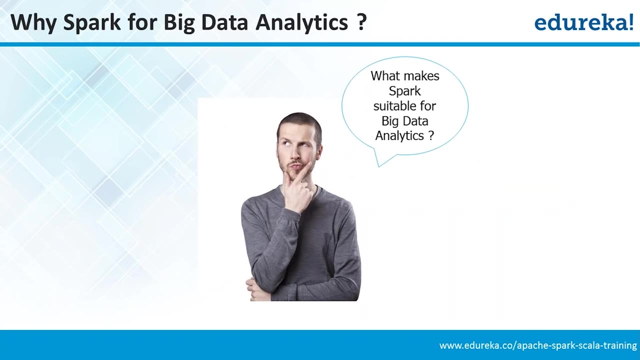 as well as other storage systems such as CSV files, Amazon S3, and NoSQL databases. So, as we discussed, it supports many underlying data sources. So what makes Spark suitable for big data analytics? So, folks, if you consider the classical Hadoop world? 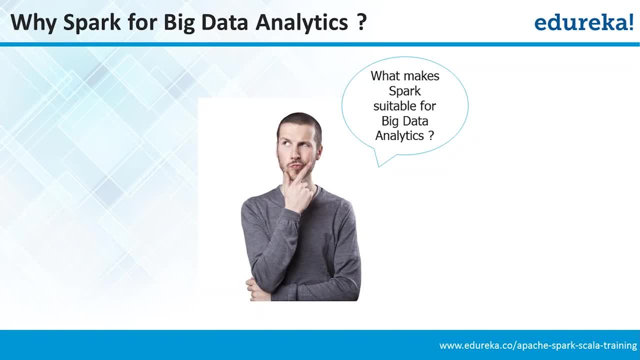 so, basically, you have got the ability to process or analyze the data via MapReduce, But with the advent of generation two, with the introduction of ARM framework, which is said to be yet another resource negotiator. So with the introduction of ARM framework, 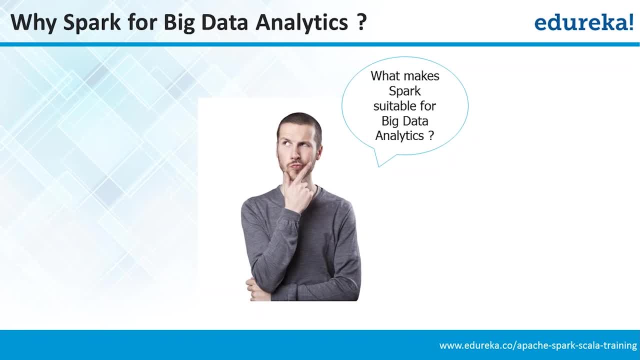 which is said to be yet another resource negotiator. So with the introduction of ARM framework, which is said to be yet another resource negotiator. So with the introduction of ARM framework, even though Hadoop opens up the channel for multiple types of applications to run on top of Hadoop. 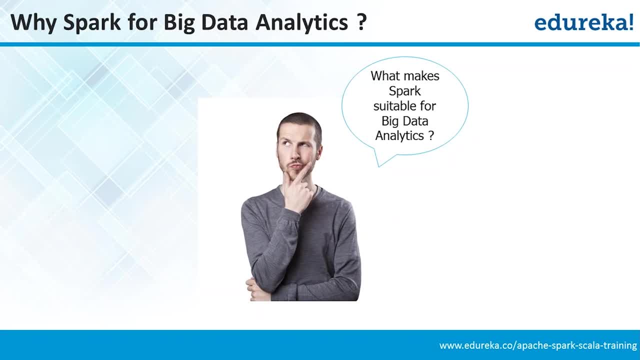 other than the MapReduce. MapReduce just become the part of it, So it actually ARM actually allows you to run other types of workloads, like graph processing applications, or say streaming applications, or say messaging applications, So different types of applications are now supported. 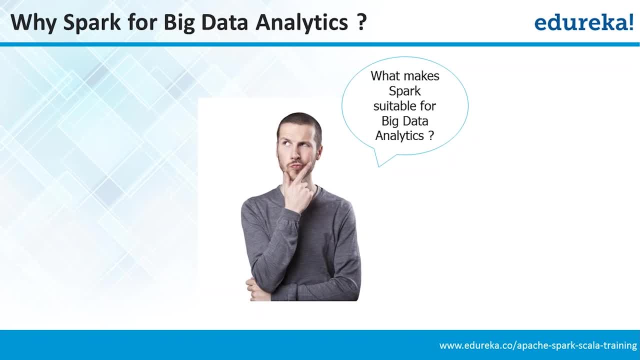 on top of Hadoop and makes Hadoop still to continue in the open source world. So okay, so now that we have got ARM, now that ARM allows you to run different types of applications on top of Hadoop, then why we are saying that Spark? 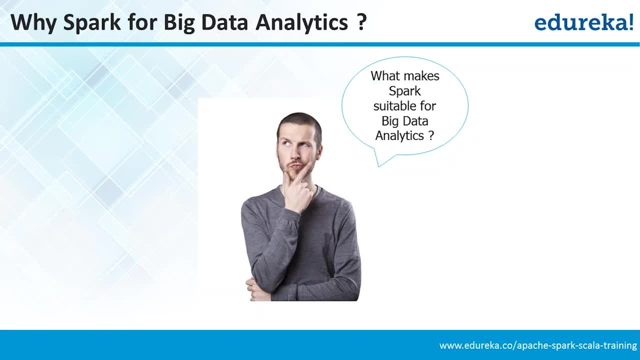 is most suitable for big data analytics. It has an interesting discussion here. So Spark is not only about MapReduce folks. So keep in mind that Spark has got different modules which are packaged in a single framework called a Spark. So what are all those other modules? 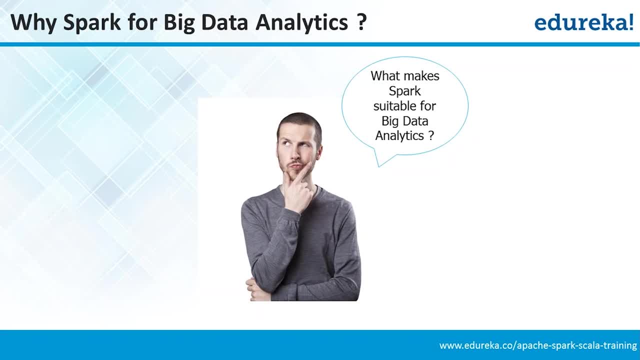 which are actually packaged as part of the Spark. Spark MapReduce is by default, and then Spark's Graphics, which allows you to write graph-specific applications on top of Spark. Spark Streaming Module, which allows you to integrate streaming applications with Spark quite easily and efficiently. 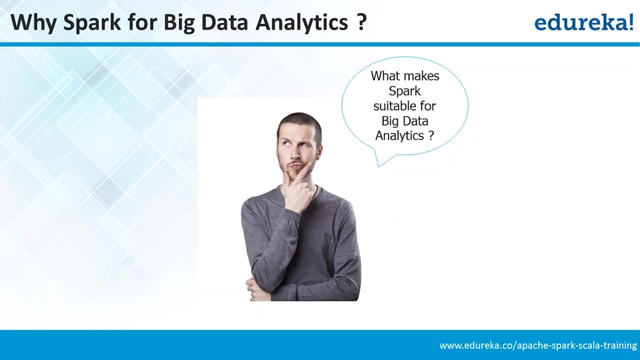 Even though there is slight difference between other streaming applications and Spark Streaming Module, which I will. I'll discuss about that in a moment. So Spark Streaming, Spark Graphics, Spark MLlib- MLlib package is another the most prominent framework nowadays because of the adoption. 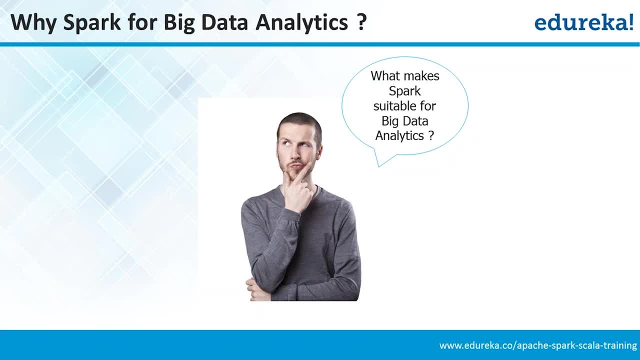 and because of the number of algorithms being implemented in Spark's MLlib mission learning and the number of applications being implemented in Spark's MLlib package. So then, finally, last but not the least, Spark SQL, which allows SQL developers to quickly able to analyze. 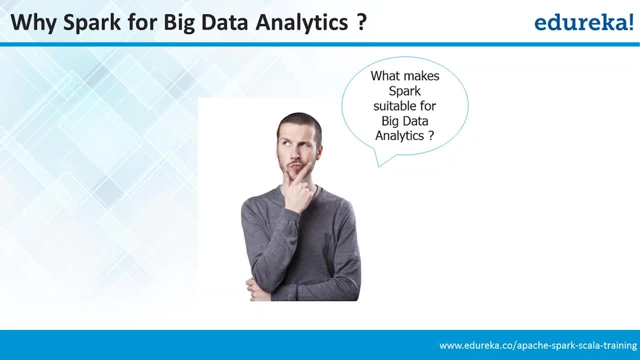 the massive data set sitting on top of any data source via the Spark SQL quite quickly or quite efficiently. So these are different modules bundled together as a single framework. So how does it matter? So how do having an in place supporting all types of applications? 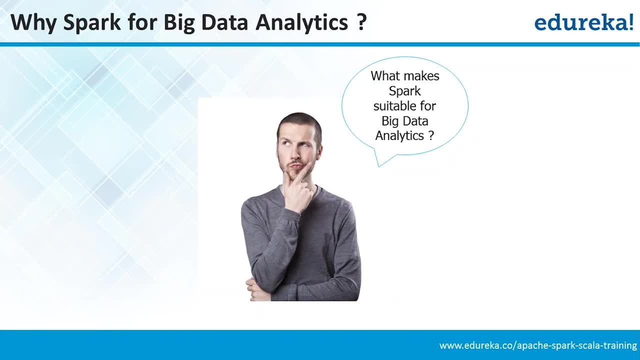 On the other hand, Spark being a single framework, having all types of workloads integrated together, how does it matter to a developer, to a company? It's very, very crucial to understand. So, folks, for you, you'll no need to learn multiple. 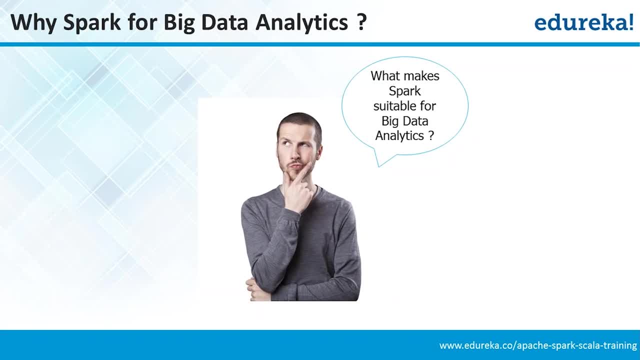 so expand your experience. You won't need to worry about other frameworks lying around the Hadoop ecosystem, Just for example, if you want to do Spark SQL programming or if you want to do graph analysis, if you want to do, if you want to apply. 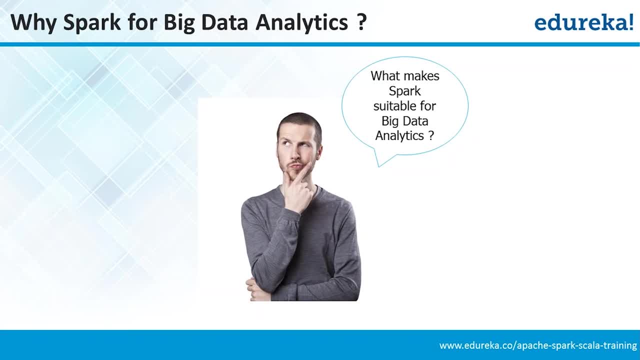 most complex mathematical models, If you want to say, for instance, process the streaming data. so you don't need to learn multiple technologies. You don't need to worry about how to integrate multiple technologies andえる those technologies with your Hadoop platform. 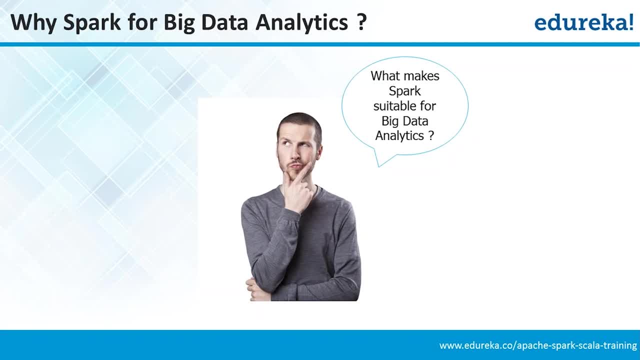 to be able to seamlessly work for you. So that's where Spark gains even more popularity. So you don't need to learn such different frameworks. rather, you just learn single framework called a Spark. So you are done. so you'll be able to run. 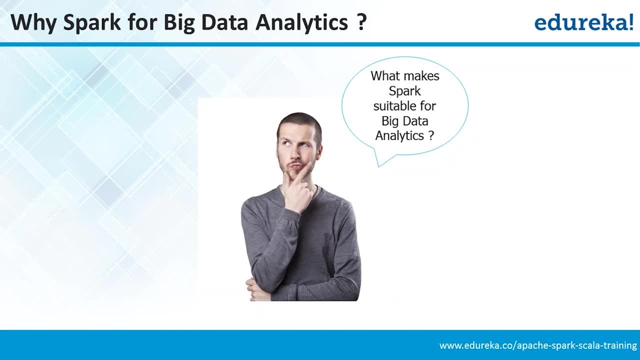 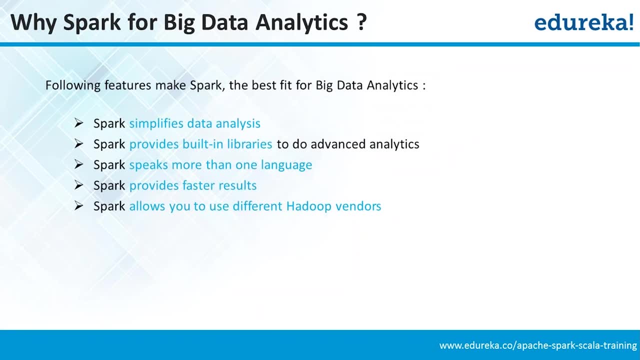 any of these types of workloads because of all these modules being bundled together as a single framework. So let's move on and see some other aspects of Spark. So Spark simplifies data analysis, So we will see. so this is also very, very important. 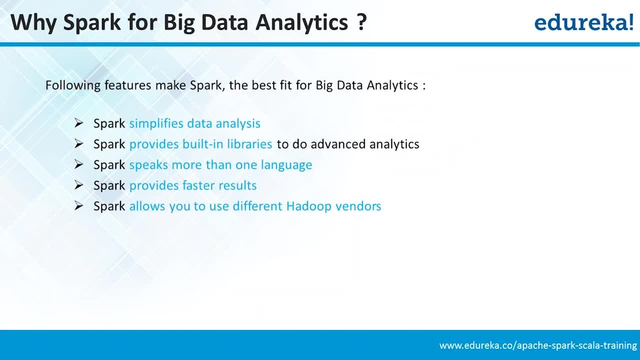 to understand folks Why it simplifies data analysis. It's because the next couple of slides will give you a very good understanding on why it simplifies the data analysis. For example, Hadoop's MapReduce being the job of the Spark framework, you have to write tons of lines. 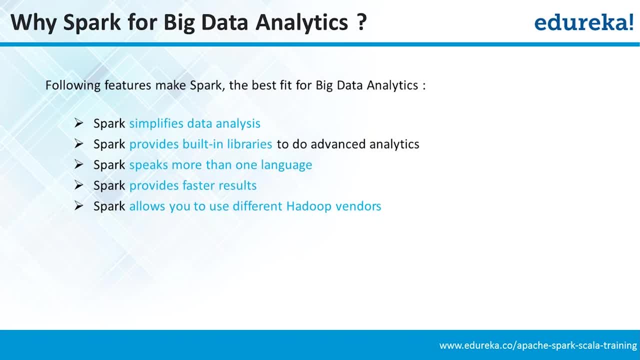 of code to implement simple application in MapReduce in Hadoop's MapReduce. On the other hand, Spark being implemented in Scala. Scala is the language in which Spark framework has been built. it allows you to implement complex applications in very few lines of code. 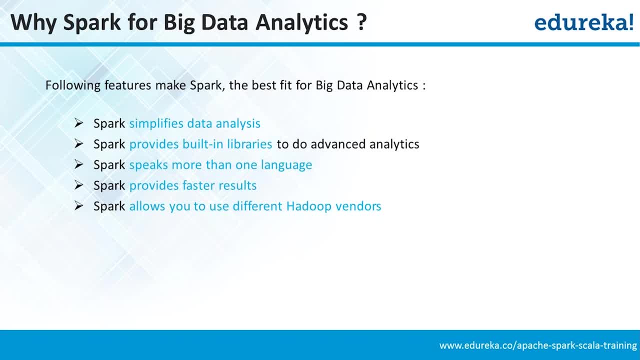 Especially because of its scalable computing capabilities that Scala provides. So that's the key differentiator for Hadoop, MapReduce and in this, Spark's MapReduce. So I'll show you. I'll show you practically how many lines of codes are reduced while you implement. 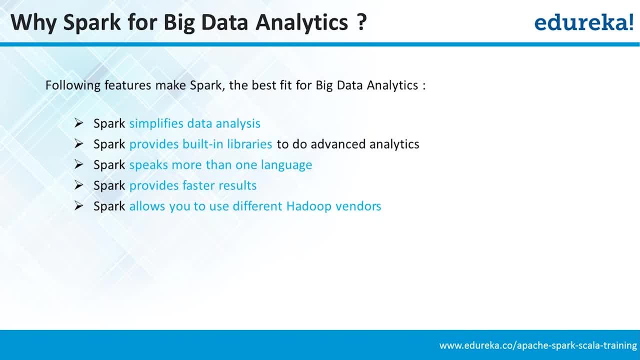 code in Spark. Then Spark provides built-in libraries to do advanced analytics. So it has got built-in machine learning library package which has got implementation for different types of algorithms, like supervised learning techniques. it has got. unsupervised learning techniques it has got. 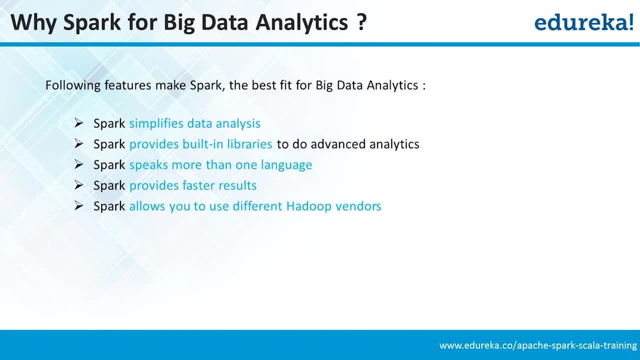 regression algorithms. it has got recommendation, information retrieval kind of algorithms And this package is growing quite quickly because of the number of developers supporting that particular package and in fact today we have got support for R as well. So not all the functions in R are supported in Spark. 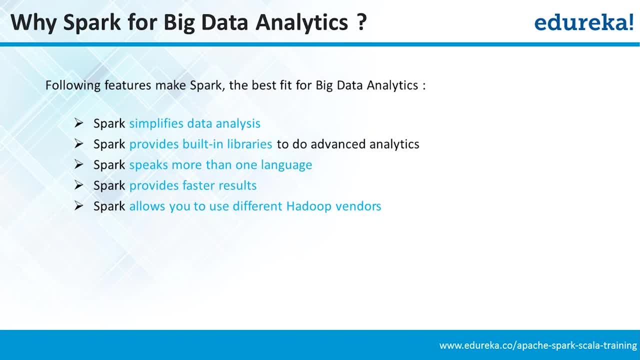 but there are quite a number of functions which are most popular, which are today supported in Spark. So then, Spark speaks more than one language. So this in the first slide. we have seen Spark supports Java, Python and even Scala. So what does this mean to us? basically, So, 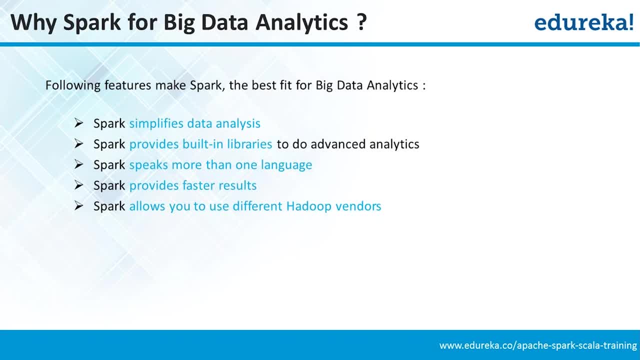 in the development community. any developer development community may not need to learn a new technology to be able to implement the code on top of Spark. Rather, they can implement in their own well-known technology, For example, say, Python. if you are a Python developer, just don't worry, just go ahead. 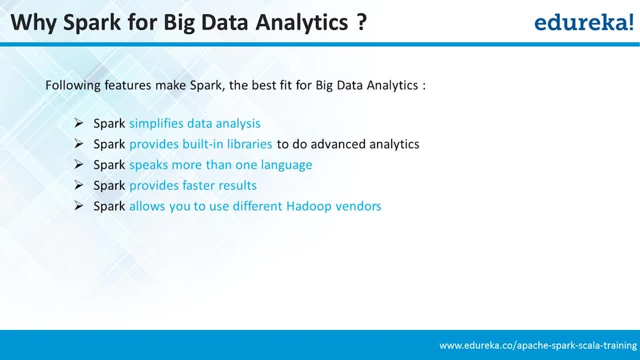 and implement your code in Python via Spark. So if you are a Java developer, just go ahead and implement your code in Java. So if you are from Scala background, so just use Scala. So it has got multilingual support, multi-language support. 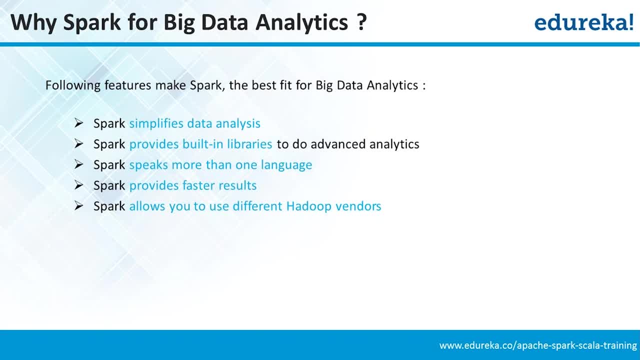 Okay, so then Spark provides faster results. So why does Spark provide faster results? It's because Spark, basically, is built around an interesting data structure called as RDD, resilient distributed data set. So this data structure, in fact I would say most of this, Spark components. 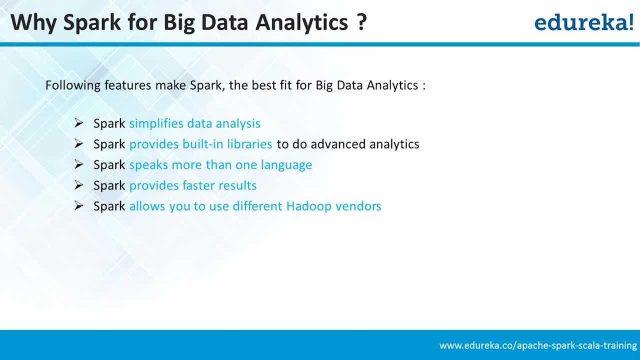 has been actually built around this data set folks, This data structure which actually allows you to load massive data set into memory with high reliability And with high efficiency as well, And a lot of other techniques actually follow that. So, because of that, because of the in-memory, 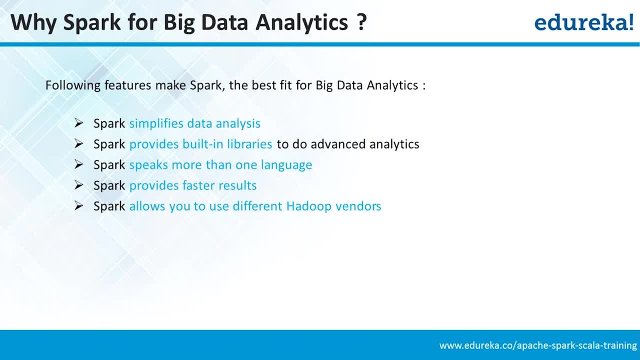 computing capabilities, Spark is quite efficient than that of any other frameworks. And then Spark allows you to use different Hadoop vendors. So, as I mentioned, Spark is not just supporting Apache Hadoop, so Spark today supports multiple third-party Hadoop. 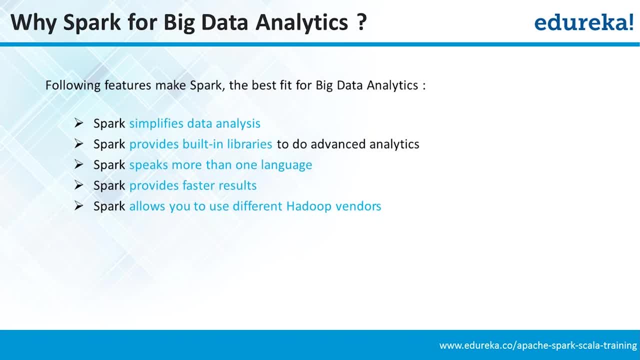 Third-party vendors available over the market, Say MapR, say Cloudata, say Hortonworks, Even say Huawei Distribution. So most of you may not be aware that there is something called as Huawei Hadoop Distribution which is available in the market. 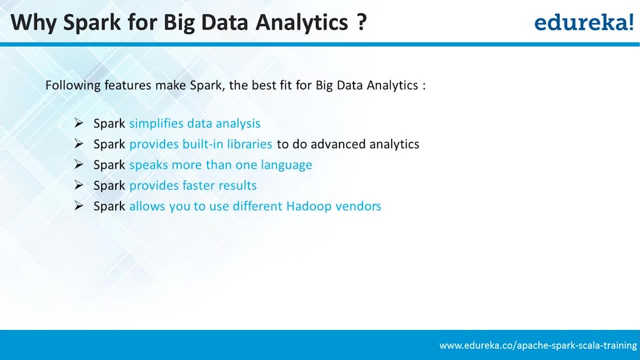 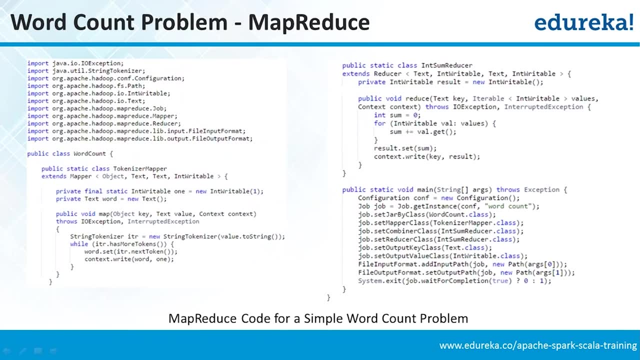 So even Spark is supported in that kind of distributions as well. Okay, so let's take a quick look About the first point which I discussed. So it is quite simple to implement code in Spark. Why? Here is one slide folks. 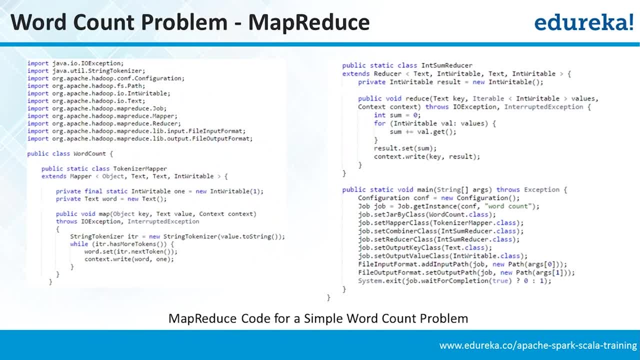 Please have a quick look on the slide. Could you tell me how many lines of code has been written in this slide? Everyone on board? So this program is basically a word count program, which is a kind of hello world program For Hadoop MapReduce. 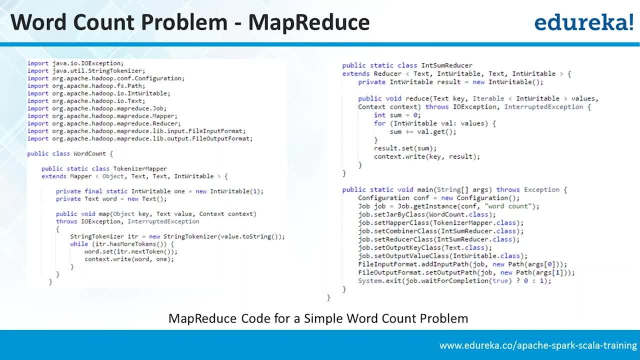 So approximately, you could imagine somewhere around like 40 to 50 lines of code has been implemented in this slide For Hadoop's MapReduce. The same functionality, the same program can be implemented in Spark. Let's see in how many number of lines in the next slide. 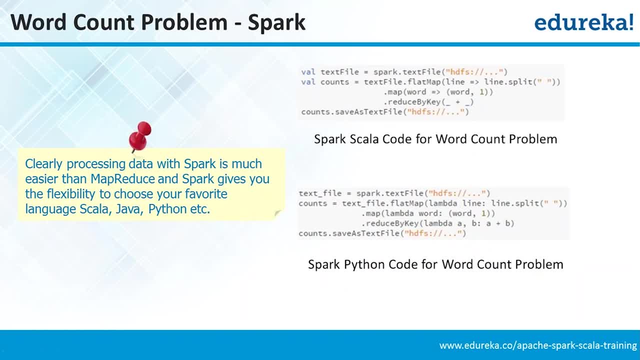 So, folks, the same program has been implemented in Spark just in three lines of code, If you look at the first three lines here. so this basically allows you to perform the word count operation in just three lines. Why is there such a drastic difference? 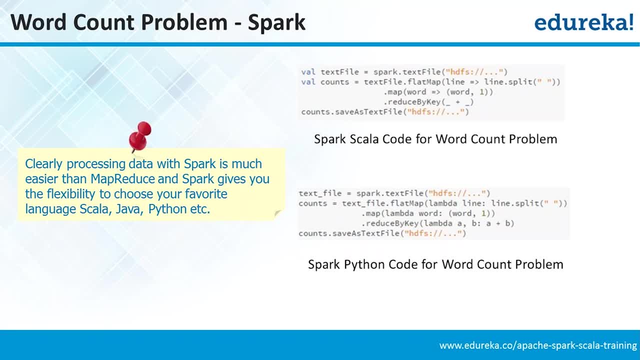 It's one of the key reasons is mainly because of the Scala programming language. So, as I already mentioned, Scala allows you to implement highly scalable code, And the development time required for implementing applications in Scala is quite quite less than compared to that of the Java programming language. 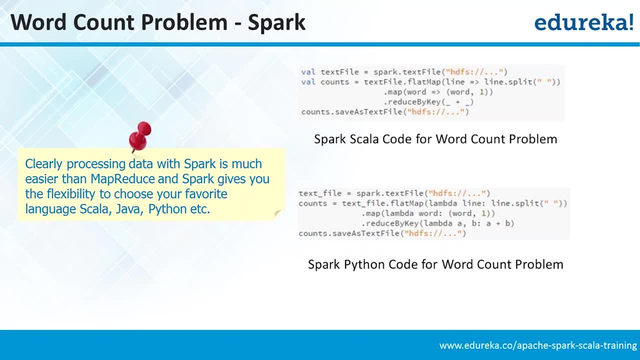 as such. Okay, So here is a quick differentiation between Hadoop's MapReduce versus the Spark's MapReduce folks. So this clearly, processing data with Spark is much easier than MapReduce, And Spark gives you the flexibility to choose your favorite language as well. 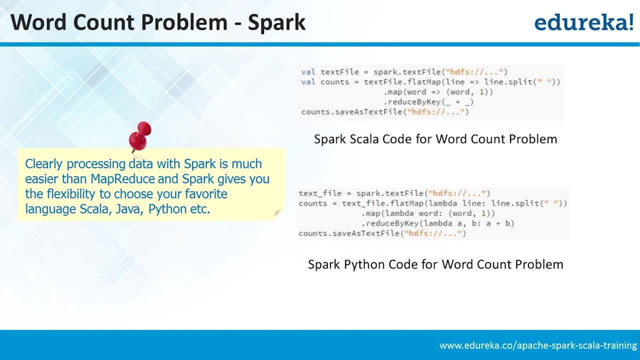 So it is not really required for you to implement the code in only specific languages- Scala or Java- So you can actually switch over any type of language depending on how flexible you are in which type of language. So, if you observe carefully, this slide, 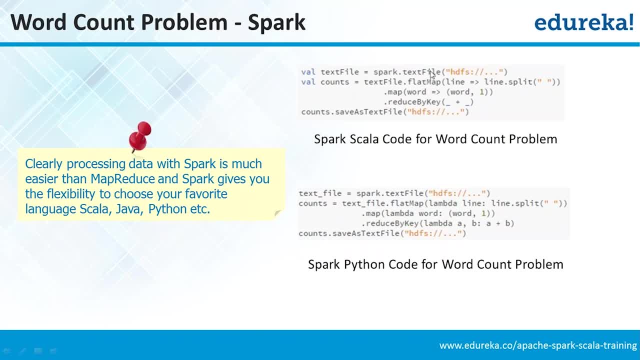 the top three lines over here has been implemented in Scala, versus the down three lines have been implemented in Python. Okay, So what I will do at this point in time. so we have been talking about too many conceptual things, So I would like to show you practically. 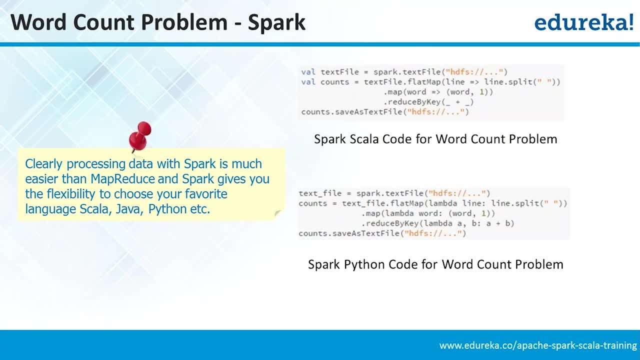 so I would like to show you practically how Spark is more efficient than Hadoop's MapReduce, how Spark is more efficient than Hadoop's MapReduce. Just quickly I'll run a simple application, the same simple word count application, on top of Hadoop. 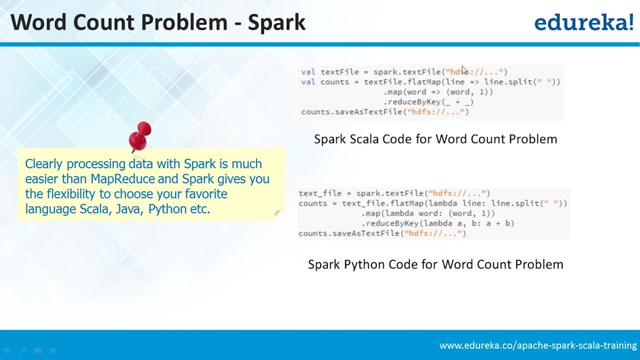 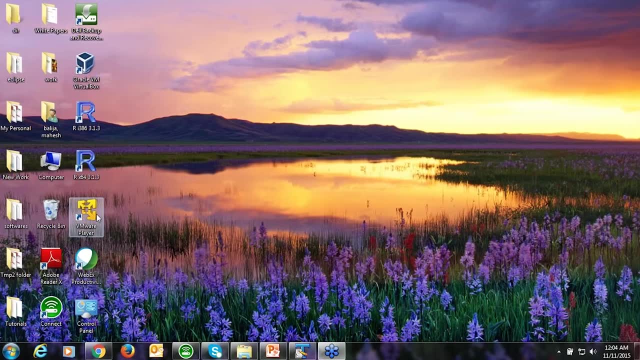 versus on top of Scala. So let's have a quick look at that, folks. So what I'm going to do here, I'll quickly run my word count. So what I'm going to do here, I'll quickly run my word count virtual machine and I'll show you the installation. 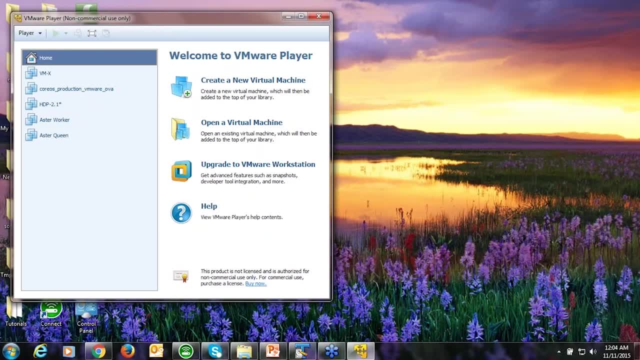 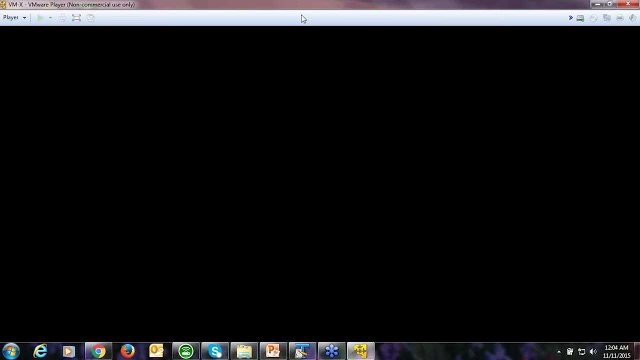 directory of Spark, or maybe I can skip that step. I can quickly start both the Hadoop and Spark clusters and then run the word count program against both these frameworks And we'll literally try to compare the performance between Hadoop's MapReduce versus Spark's MapReduce. 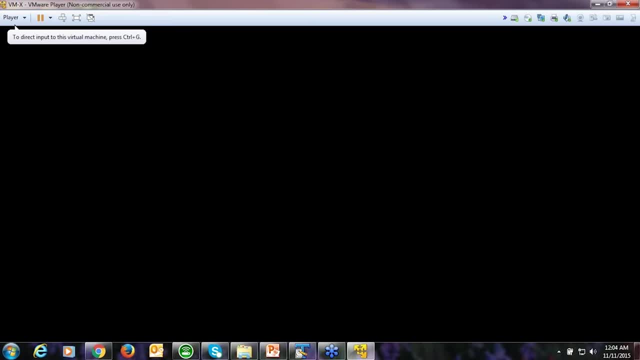 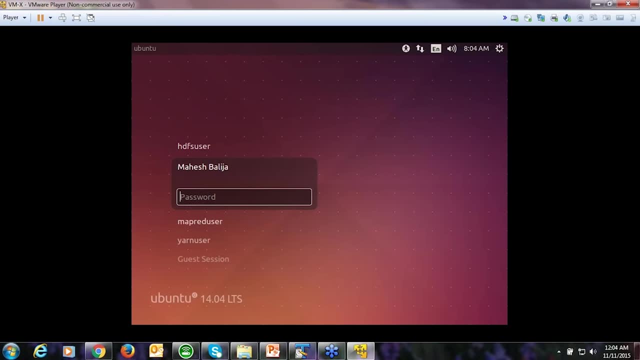 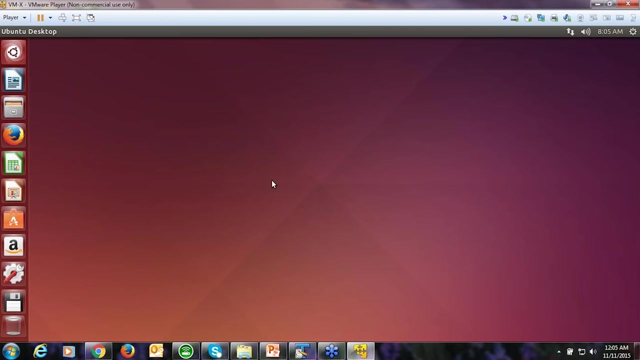 Okay, I know there are plenty of questions floating around. Please accept my apologies. all the slides- and then I'll give some time to you to ask your questions. so I'll clarify your questions, folks, in a moment. Okay, So I'm just going into my Hadoop. 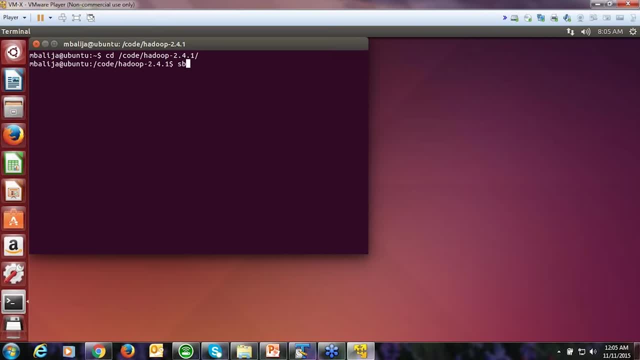 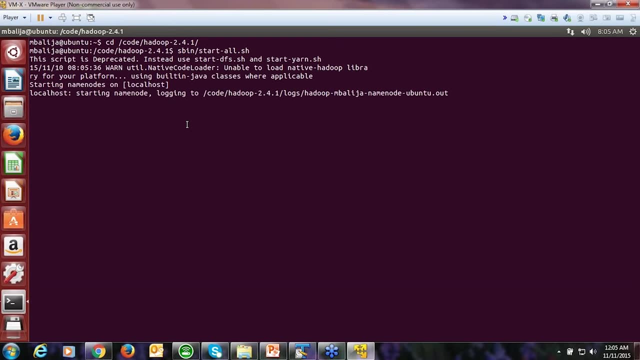 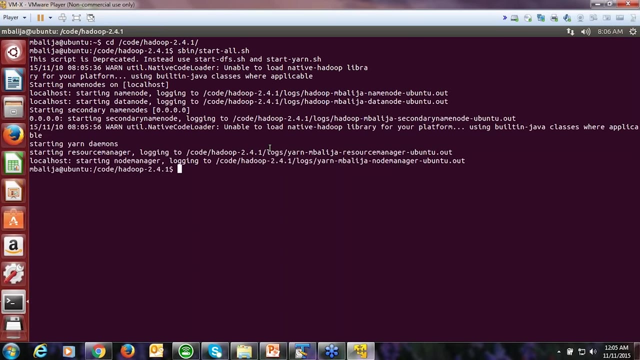 so, which is 2.4.1, and then I'll quickly start my Hadoop cluster. At the same time I'll start my Spark cluster as well. Maybe I'll take another 10 to 15 minutes to continue with the discussion, and then probably I'll give. 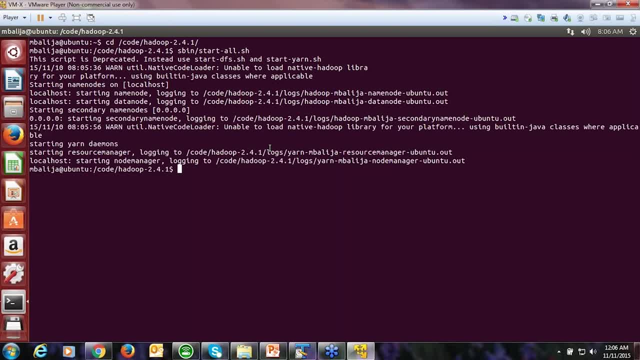 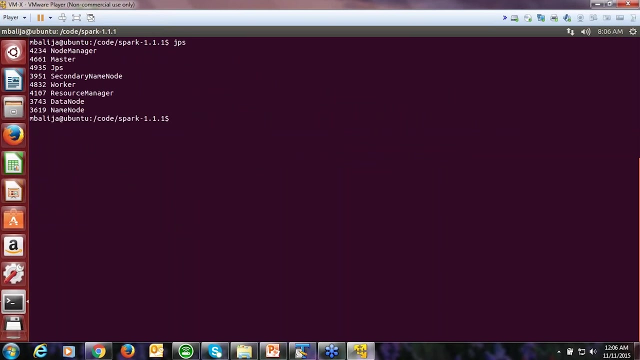 the rest of the time for the Q&A folks. So I'm starting my Spark cluster now. My Hadoop cluster has already been started so I can quickly check. I think almost all the services are running quite successfully. I can see Master Worker which are from Spark. 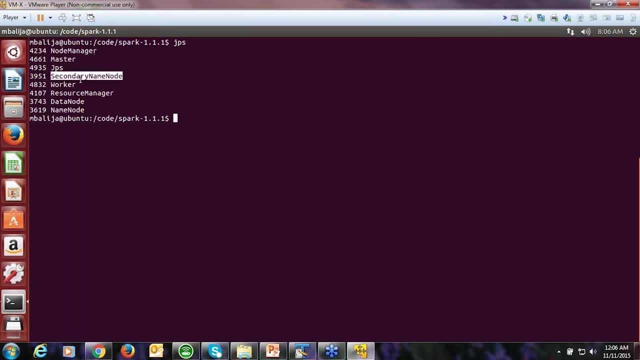 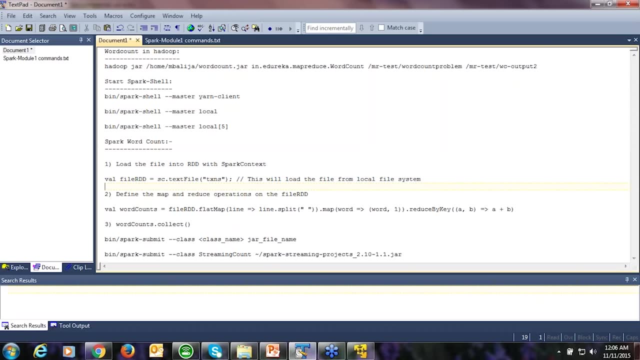 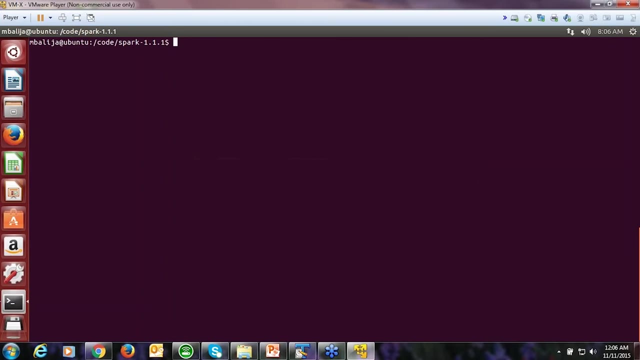 and I can see the remaining services are from Hadoop. Okay, so let me quickly run the WordCon program. So I hope everyone is comfortable and familiar with the WordCon program, right? So basically, WordCon program allows you to count the words. 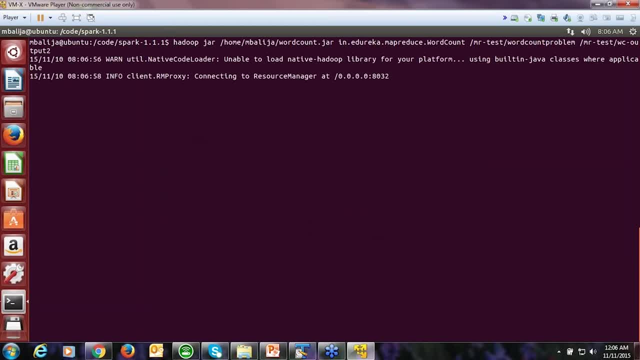 I'm sorry to count the words from the given file. Okay, so what I'm doing here is basically I'm running the Hadoop command, Hadoop jar, some WordCounter jar, and then here is my class which does the WordCounter. 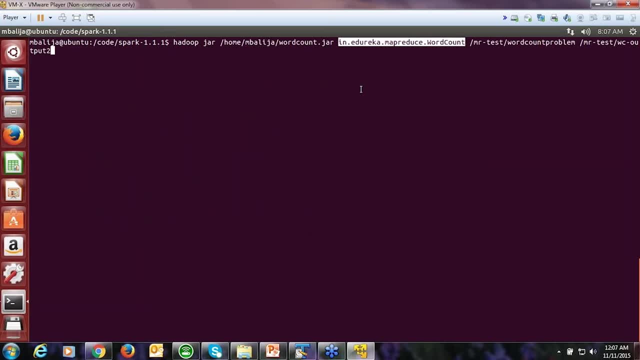 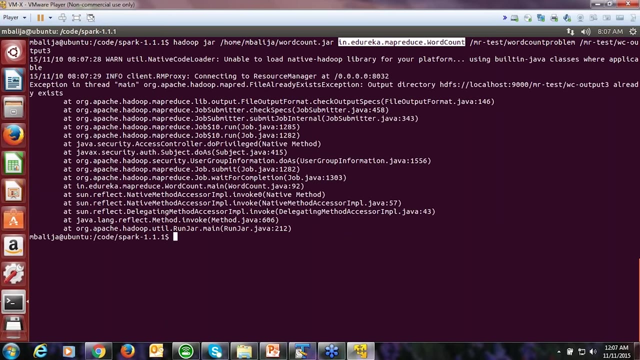 operation. just the same code. I have just put it on the slide- and then the input path and then the output path. So let me change my output paths to some other directory. So now I'm running this application to count the words. to count the words. 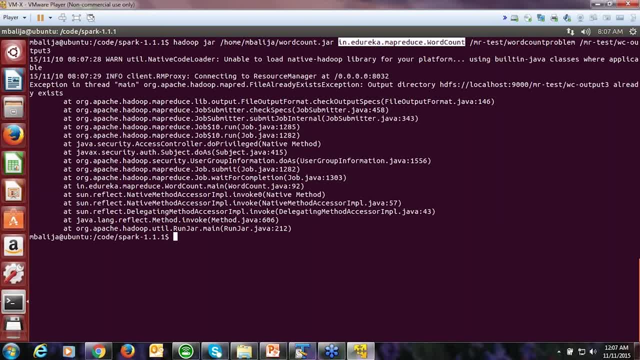 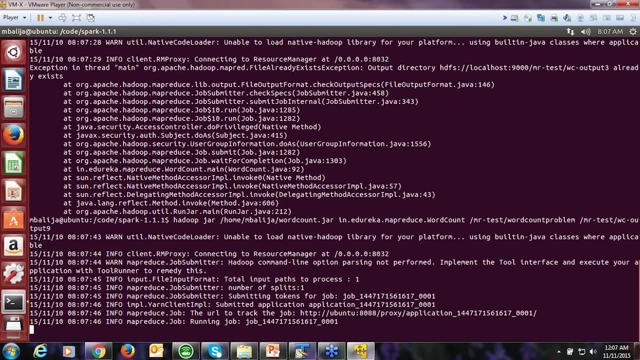 Count the words. So output directory already exists. okay, No problem, let me take another output directory. Excellent, so now my program has started running. It just complained, or it just shouted on me saying that your output directory was already existing. 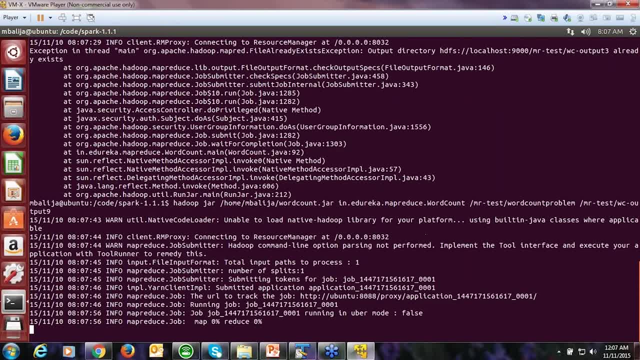 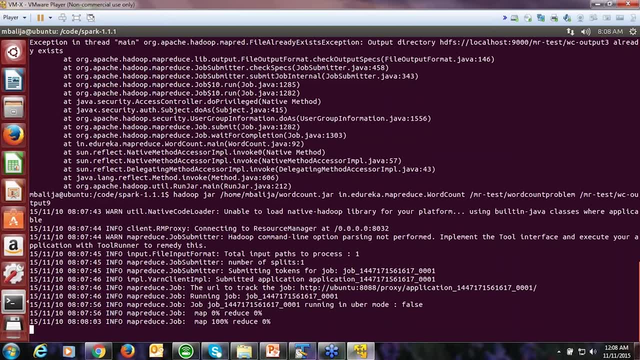 so please remove the directory. So, rather than removing my output directory, I have specified a new directory path. I think we should suffice our needs. So my mapper is. my mapper is successful, 100%. My reducer is about to start, which is still running. 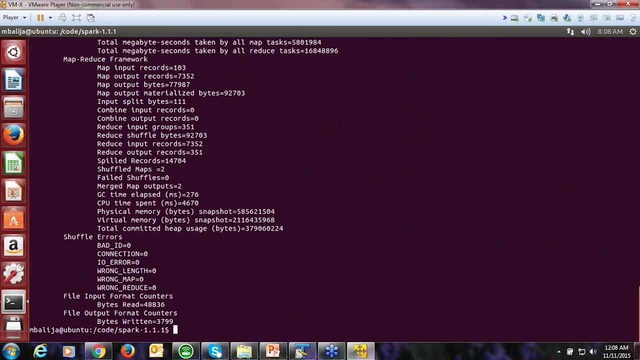 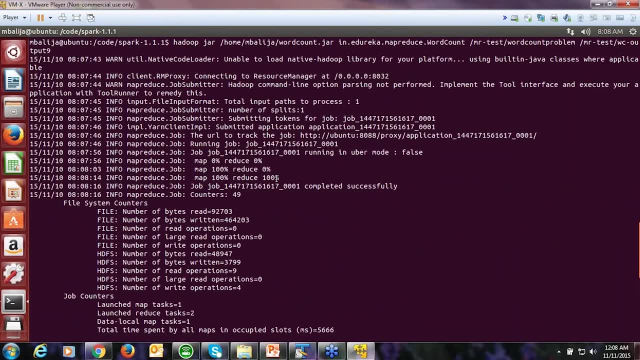 I can see it's still running. My reducer also has been successfully executed. So, folks, if you carefully notice how much time this application has taken to complete, So it's basically, this application started somewhere around, let's say somewhere around, starting from 7.43,. 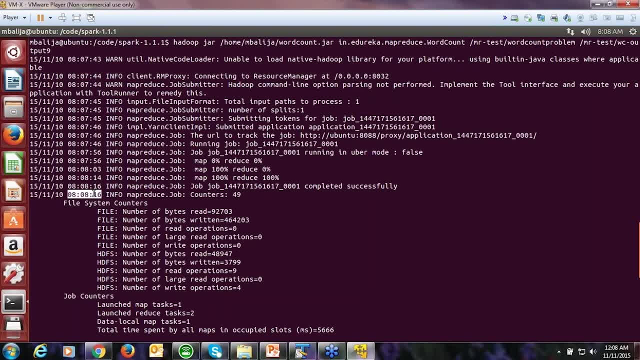 and it has completed at around like, say, 8.16, which is like cumulative, how much time it took Somewhere around 17 plus 16.. Say, approximately 33 minutes 33 seconds to complete this job on Hadoop MapReduce. 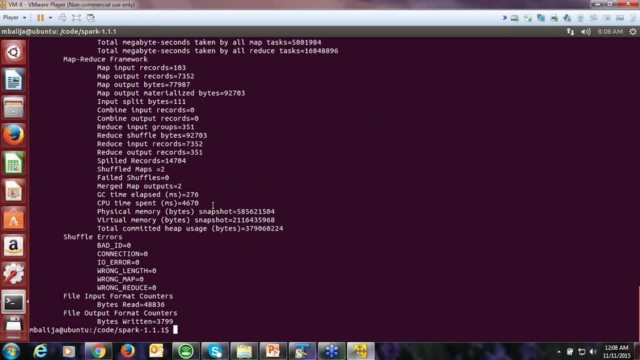 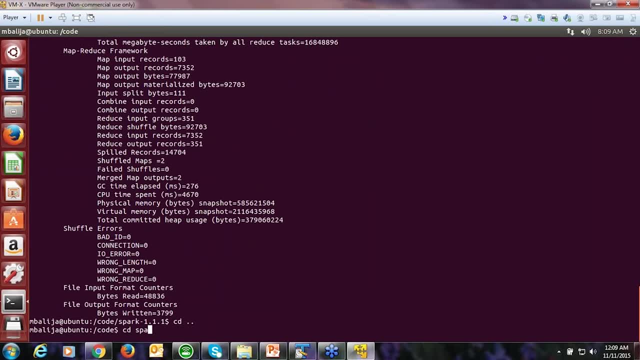 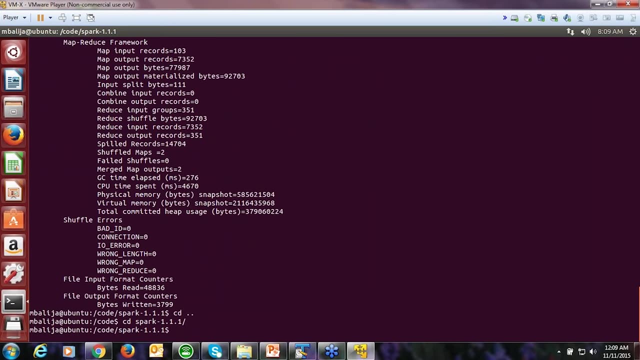 So let me try to run the same word count program in Spark now And try to compare the performance. Okay, So now Spark. another beauty of Spark is basically it has got an interactive shell with which you could interactively run your applications. 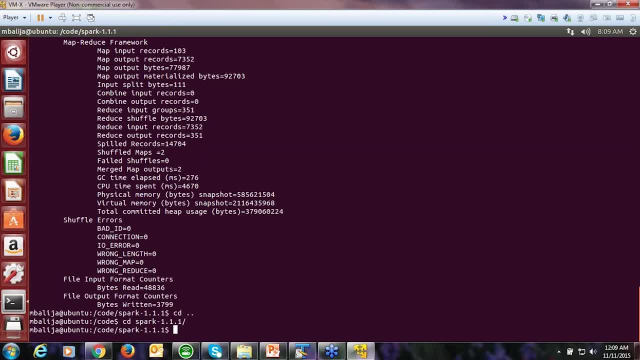 No need to run it remotely. It can interactively run your code and then quickly either load or just debug your application. folks, Okay, it is beneficial for both of these, Either for learning or for debugging your application. So now I launch that interactive shell. Okay, so with bin slash. 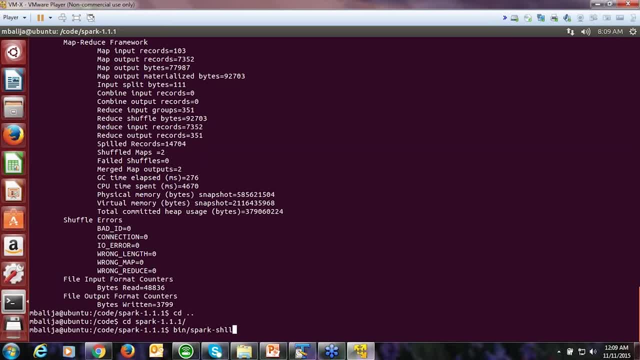 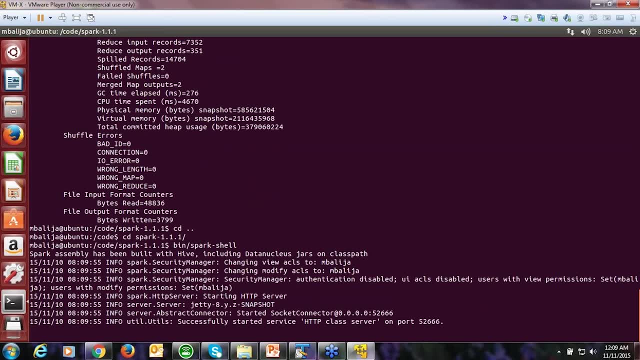 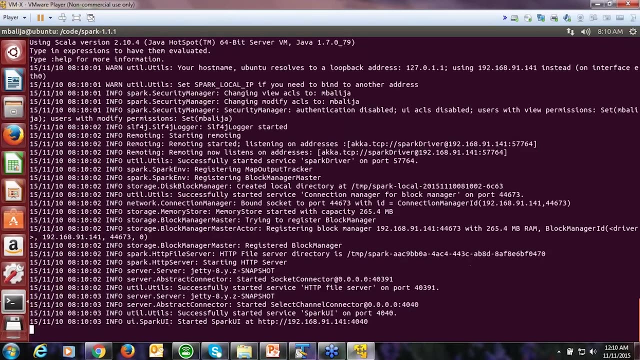 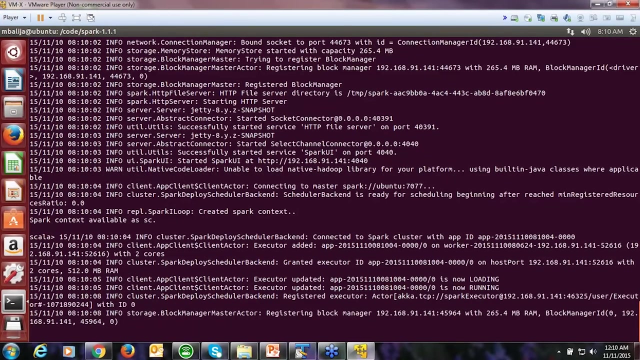 Spark shell. Okay, so now it is launching the Spark shell now. So once it is launched, I'll quickly run the program for word count on Spark. So in this case, just bear in mind one thing: That the data is being looked up from HDFS directly, And then the processing happens. 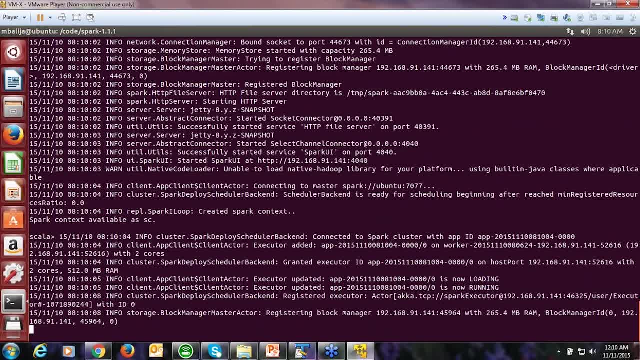 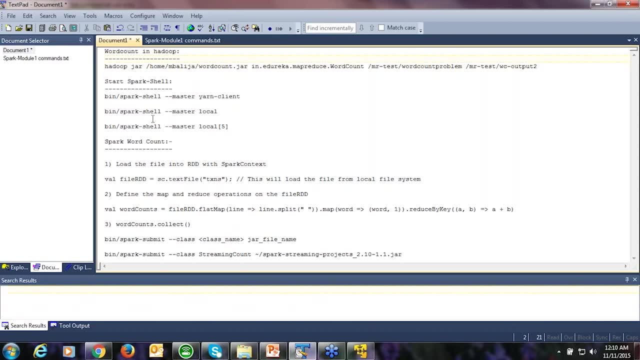 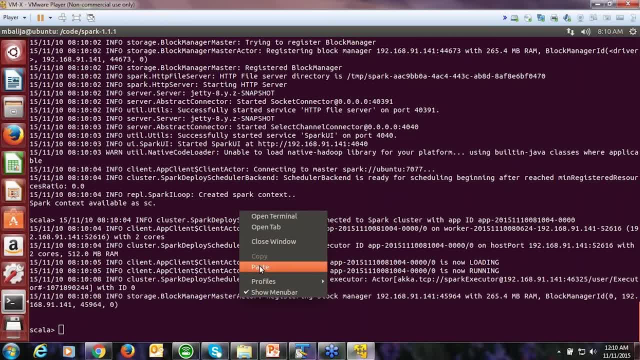 Okay, so let me actually close this one, And then I will just zoom in and see where the data is. Okay, I'm going to repeat it. So, inelそれでは. So, first of because of my, So, first of because of my. 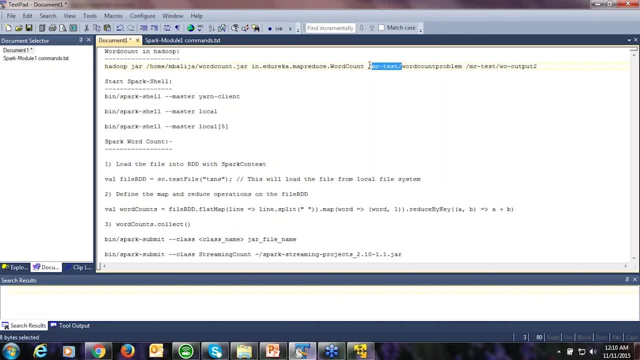 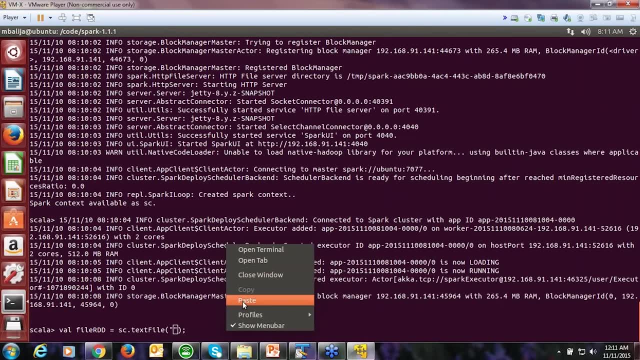 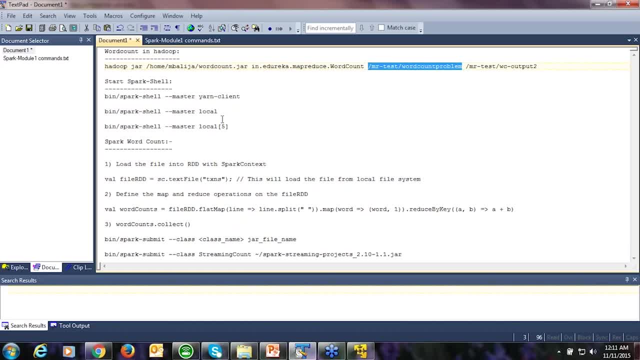 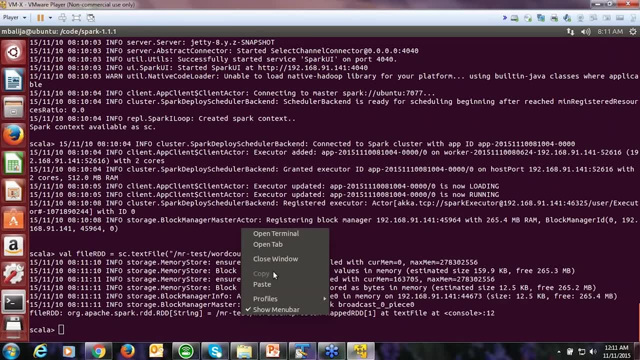 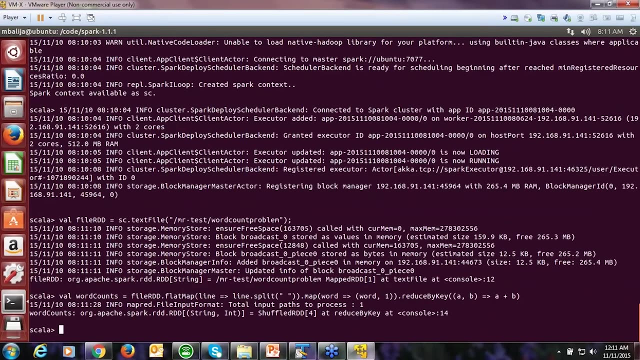 Oh, there is an error here. Click Okay, Hey, which basically does the counting of the words. I'm not going to go into the details of this, but I'll just quickly run the command, folks. Okay, so the word counts has been computed. 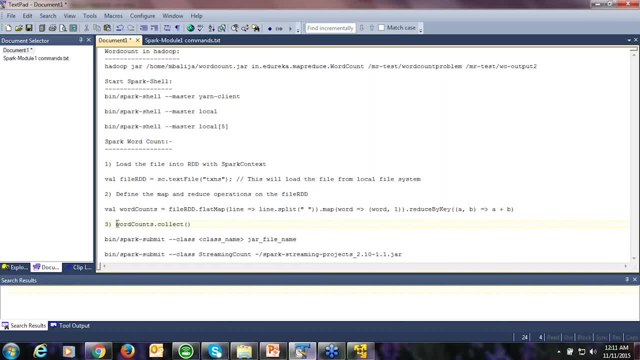 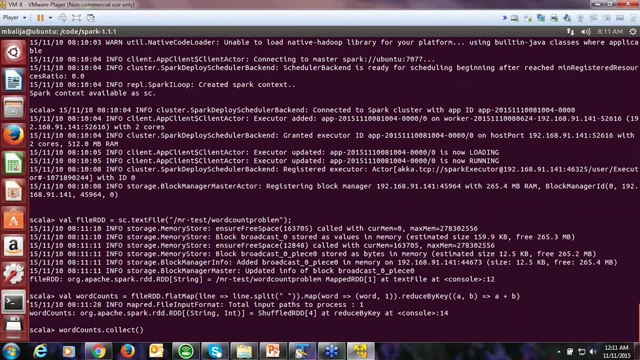 Now I'll just quickly print those word counts onto the console. Okay, so now when I run this command, it basically starts the execution. So for Scala, basically, you need to have a triggering point to kick off the project, to kick off the application. 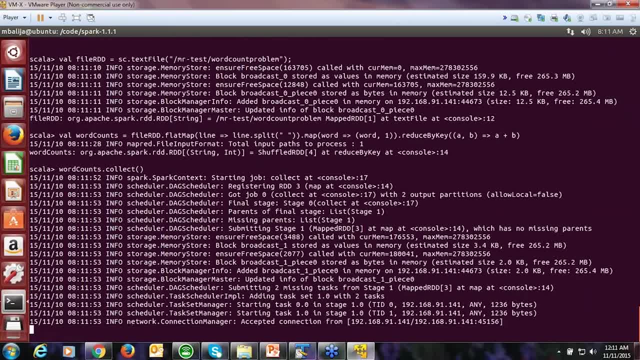 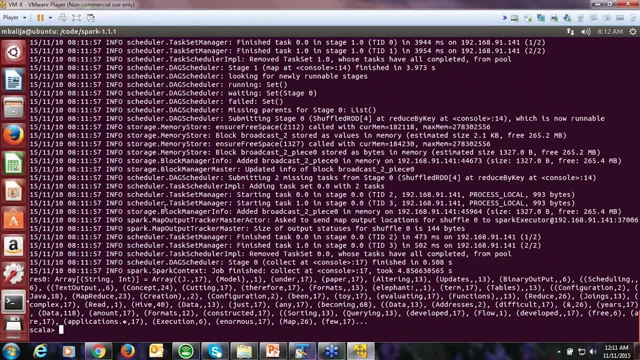 So now this command basically starts the application and let's see how much time this is going to take. Okay, so essentially, if I carefully notice, even from the beginning, which is 1152, till the end, 1157.. 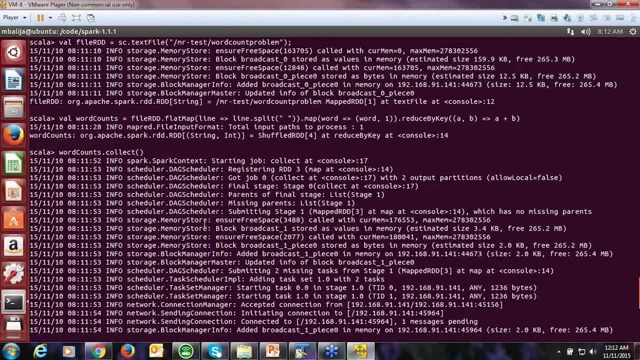 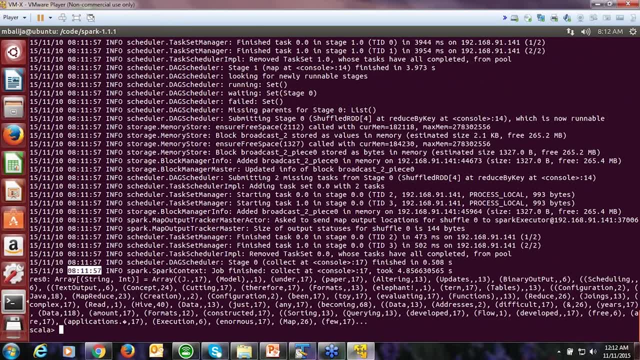 So how many seconds it has taken folks? Approximately five seconds. So this basically tells us practically that the performance of Spark MapReduce is way higher than the Hadoop's MapReduce framework. Maybe this is very, very small. so you might ask me, why do you really care? 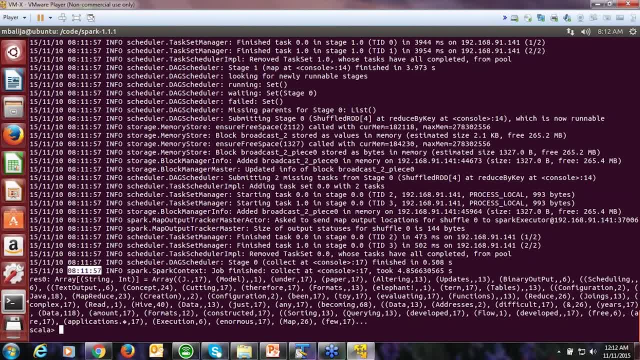 about 30 seconds versus, say, five seconds. Does it really impact anything? from your side? No, but you should think about this in the terms of highly scalable applications or high-scale datasets, where you're talking about terabytes. Then the amount of time taken will become quite significant. 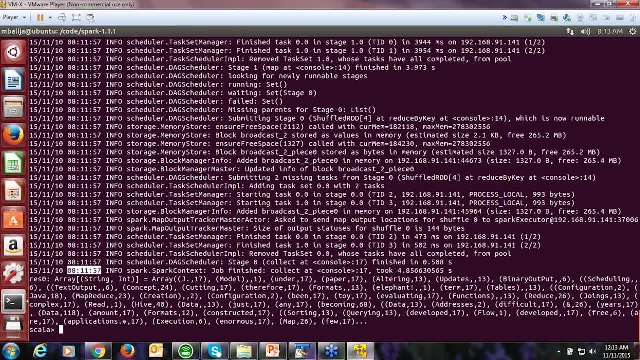 to meet the service level agreements defined by your business users. okay, So again, I don't want to again to actually leverage. use too much of business terminology here. Here the intent is to show quickly the difference between these two frameworks. 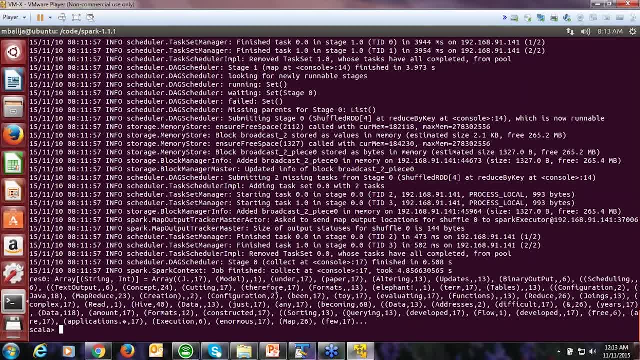 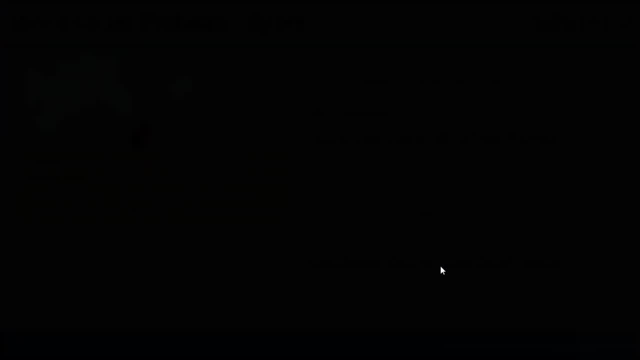 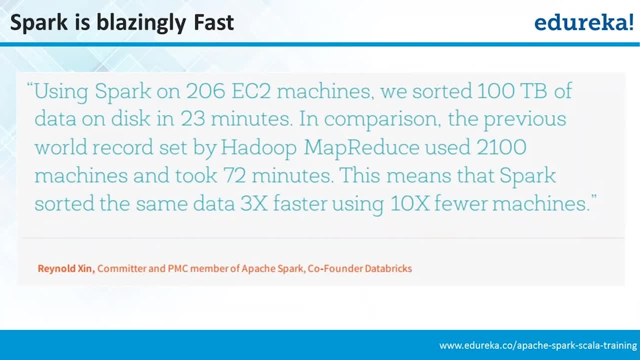 Okay so let me come back quickly and see what else is reminding for today. Okay so, folks, Spark is blazingly fast. We have seen that, In fact. here is an example. Just have a quick look around the slide. It says that, using Spark on two nodes- 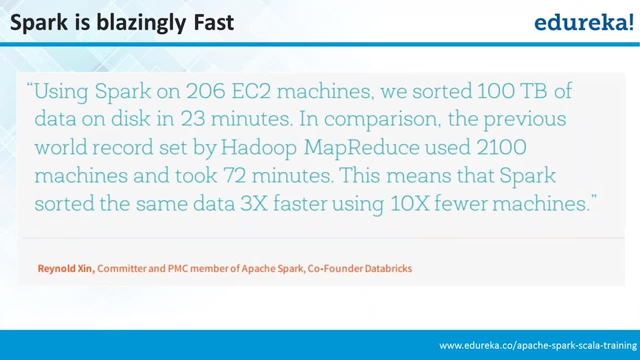 4.6 EC2 machines, Amazon Elastic Compute Cloud machines. we saw that. who is that? It is basically Reynolds and Comete, whatever PMCs from, but Spark, co-founder of Databricks, So it's basically Databricks- was able to sort. 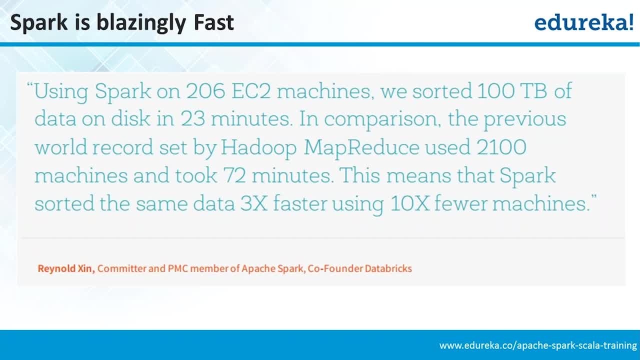 Databricks is basically the key contributor behind the Apache Spark framework folks, So they are able to sort 100 terabytes of data on disk in 23 minutes. In comparison, the previous world record set by Hadoop's MapReduce used 2100 versus 206 machines. 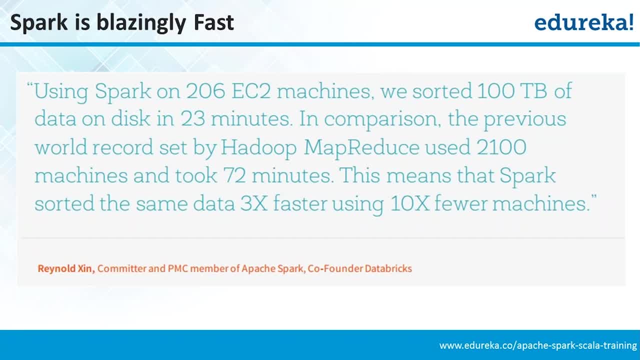 and took 72 minutes. So previously Hadoop MapReduce took 72 minutes on 2100 machines, versus today's park took only 23 minutes, which is maybe somewhere around two by third of the time. and look at the number of machines, It is nowhere comparable, maybe somewhere one by 10th. 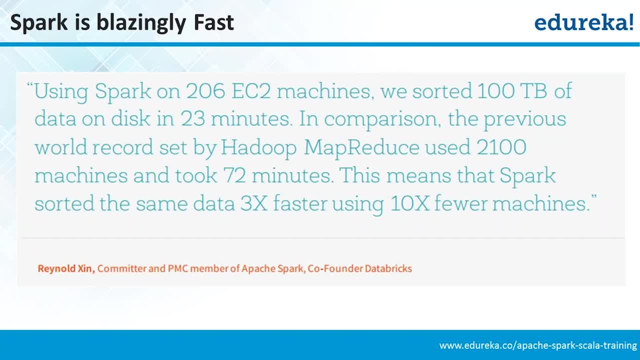 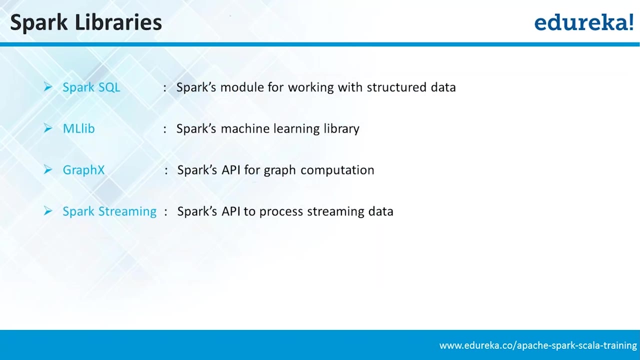 I think. less the node, less number of nodes. This means that Spock sorted the same data three times faster using 10 times fewer machines. okay, So that's quite intuitive, right? And then Spock SQL. So here are the different modules. 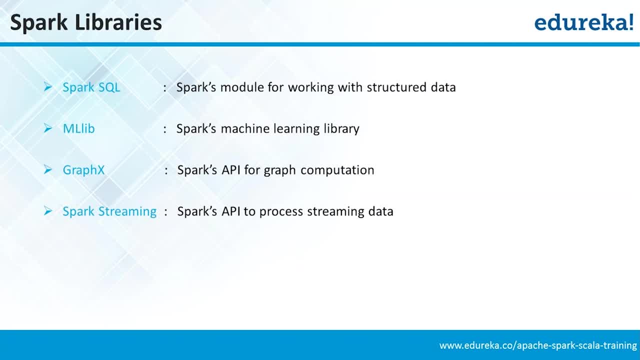 which we have already discussed. Spock has got different packages when it's Spock SQL which allows you to quickly run SQL queries on top of Hive. So basically you just leverage on the Hive metadata which is on Hive Metastore and then just runs the queries. 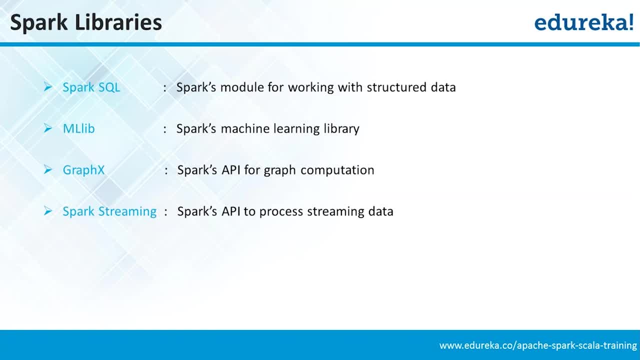 on top of Spock, to which you could analyze the Hive data, Then even HDFS data, Then MLlib basically allows you to run any complex mathematical model quite quickly and efficiently. Even developers could be able to easily learn and run the complex algorithms on massive datasets folks. 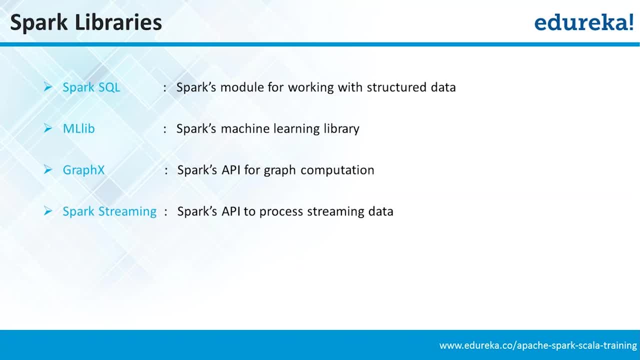 So you don't need to be really a data scientist by nature, but if at all you are just from development background. still, you are able to use those algorithms quite quickly. So learning curve is quite less, even in MLlib. Then graphics, which allows you to run the graph analysis. 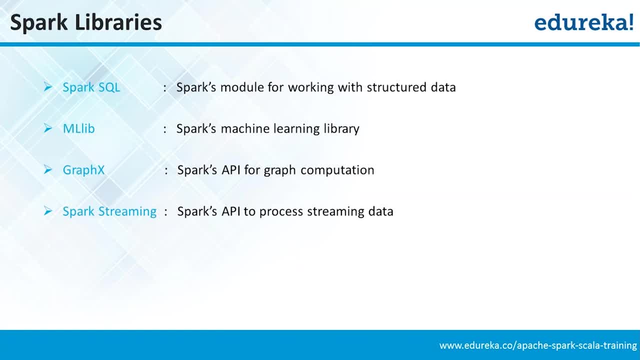 on top of Spock, then Spock streaming. So here is what I would like to differentiate between the original streaming applications, between Spock streaming. So the quick difference is, if you are talking about Storm Framework, which is quite well, quite familiar as the streaming application, 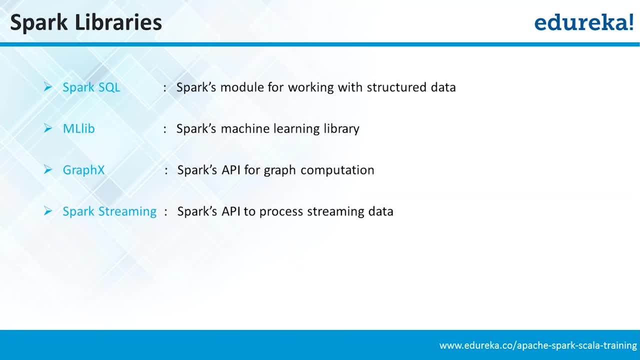 streaming framework. yes, it is true, Even today. So at a sub-second or even at a micro-second level, you could process the data using Spock streaming- Sorry, my apologies- with Storm Framework, At a micro-second you could process the data. 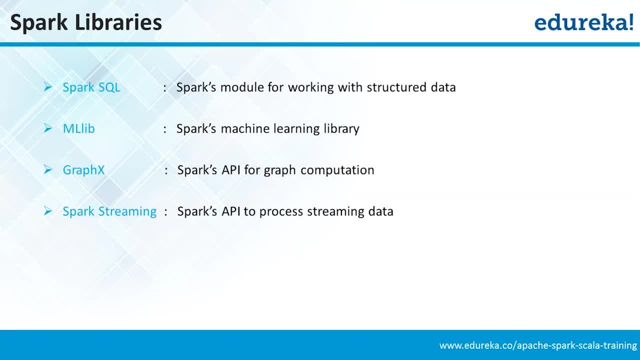 The moment the record enters into the system. you could analyze that record with Storm Framework, But with Spock streaming framework there is a slight difference, which basically allows you to streaming in mini-batches. The mini-batch could be as less as 30 seconds. 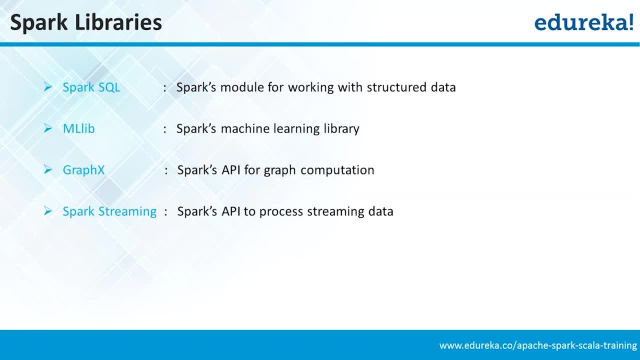 or 15 seconds, but still it is a mini-batch system. It's not a pure streaming application, Because folks bear in mind one thing: there are many applications which require you to process the data at a micro-second level. So that's the difference between Spock streaming. 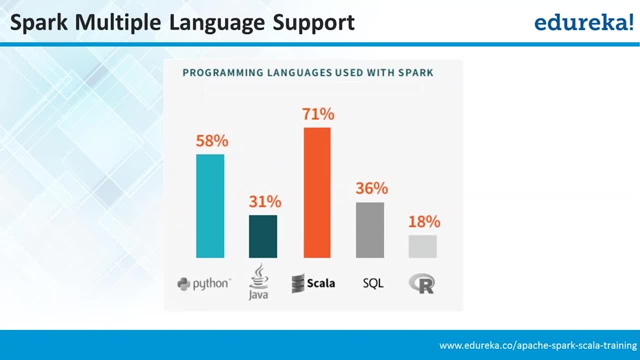 and other streaming applications, for example like Storm. So then Spock multi-language support. Here are different languages in Spock: Python, Java, Scala, SQL and R. So you can see the adoption of these languages. So, basically, Scala has got the higher adoption. 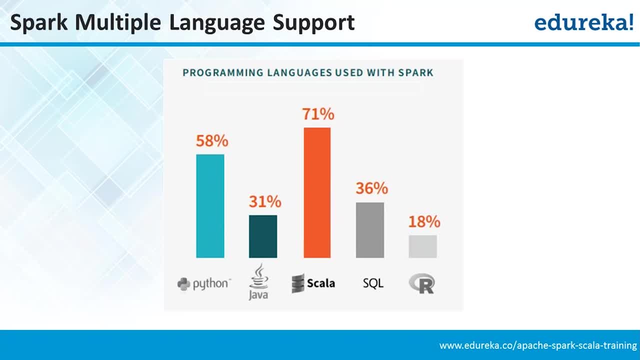 Few questions. I have seen which language has got higher adoption: 71% is in Scala, 71% is in Scala, 71% is in Scala, Java is 31% and 58% is in Python. It basically depends on how many number of users. 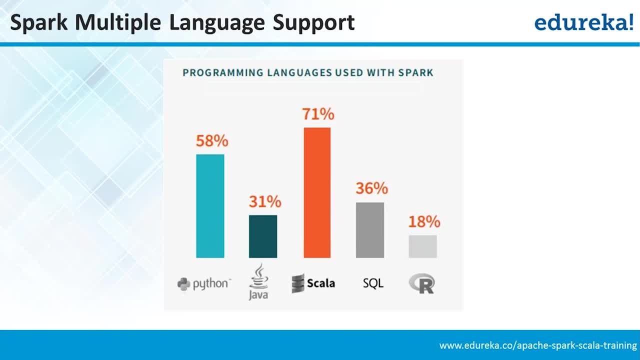 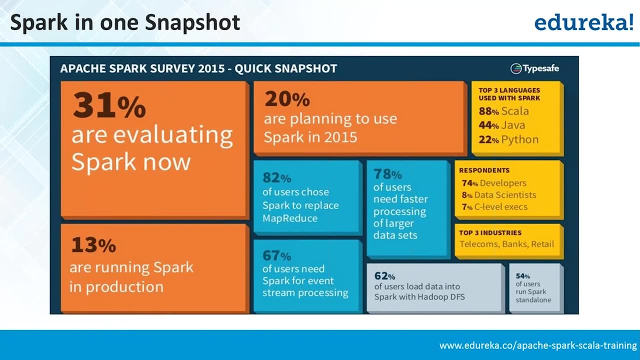 are out there who wanted to use Spock And then SQL also, then R as well. So here is the fantastic slide. throughout this PPT, I like this slide the most because it gives a very detailed understanding on how Spock has been exploited today. 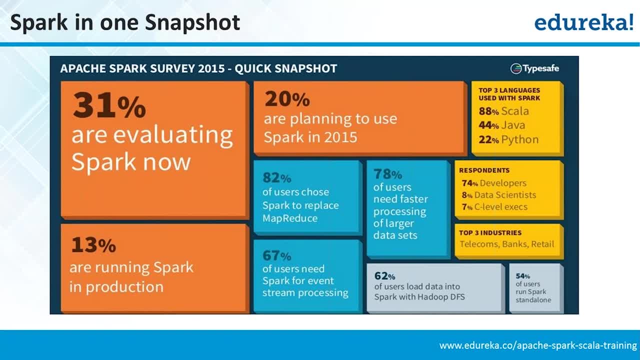 Apache Spock Server 2015.. 31% are still under evaluation phase. That's really good folks for all of us, Because whoever want to step into Spock framework say yes, just be assured that your carrier is quite secure, especially because of the adoption of Spock. 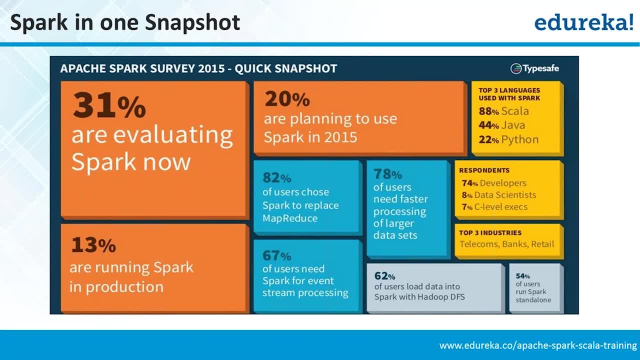 today in the market, And then 20% are planning to use Spock already in 2015.. 13% are currently running Spock in production. They are very less so it's really good to us to know. Then 82% of users choose Spark to replace MapReduce. 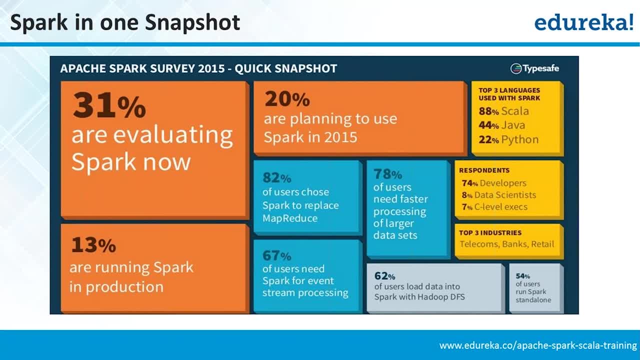 That's already we discussed and we have seen the difference. 67% of users need Spark for event stream processing. That's also a good point. You can see how crucial it is to even support mini batch kind of application. Then 78% of users choose Spark to replace MapReduce. 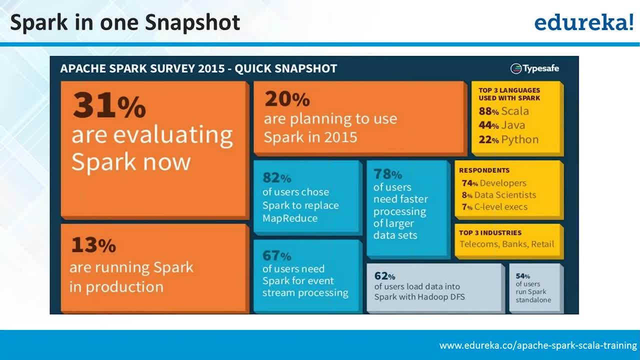 That's already we discussed and we have seen the difference. And then 72% of users need faster processing of larger data sets, So that's quite intuitive as well. Then 62% of users load data into Spark with distributed file system. So here are some more interesting topics. 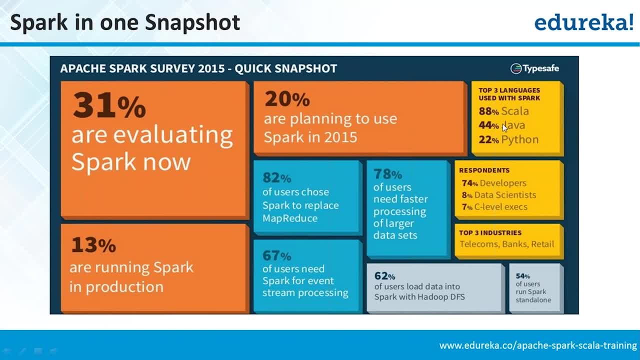 like Scala has been adopted by 88%, Java by 44% and Python by 22%, So the language is being used. so this is very, very interesting and it's very good and it's a really good idea. It's a really good idea and it's a very good idea. 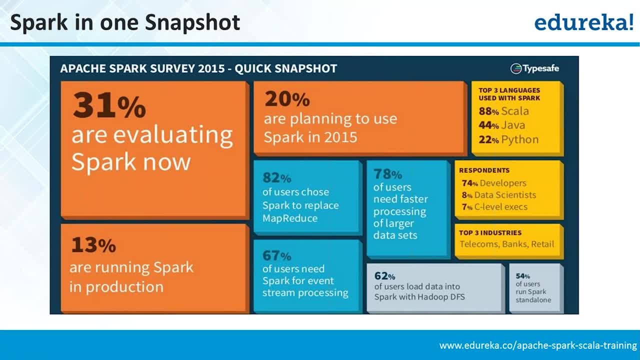 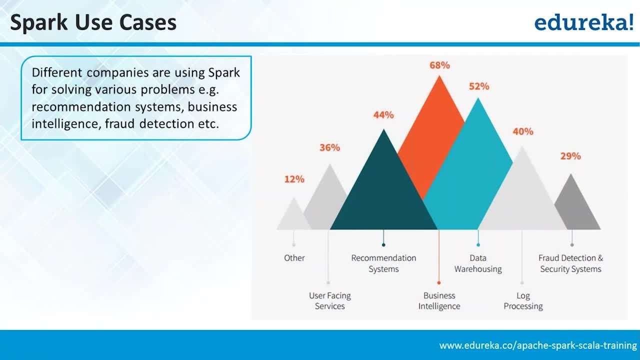 So just go through the slide whenever you find time. You'll definitely get a very good idea. So I don't need to really go through into each one of this. So Spark use cases. Different industries has got different applications for Spark. different usage scenarios for Spark. 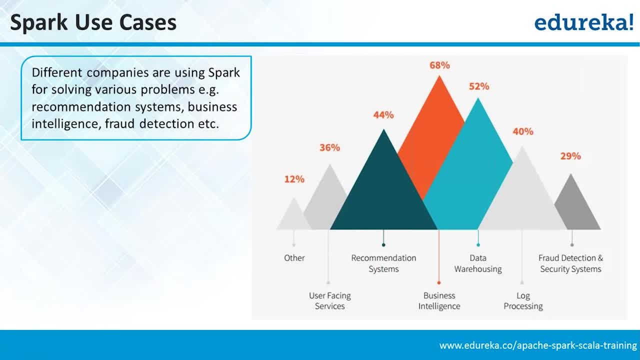 However, Spark is used for resolving various problems like recommendations, then business intelligence and fraud detection, detection, So when I say recommendation, so basically, Spark has been leveraged as a machine learning tool for analyzing large data sets, So that's one of the key applications via the machine learning library package. 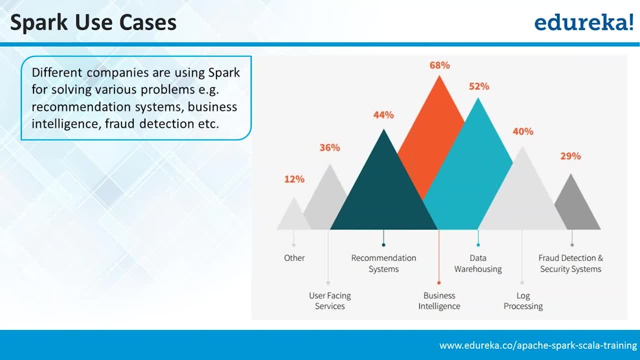 Business intelligence application. so basically, if you have got visualization tools, for example, like say Tableau or say MicroStrategy or any other BI tool, basically you can easily integrate the BI tool with the Spark framework via Spark SQL or any other module. Fraud detection- so again it's a machine learning specific use case. 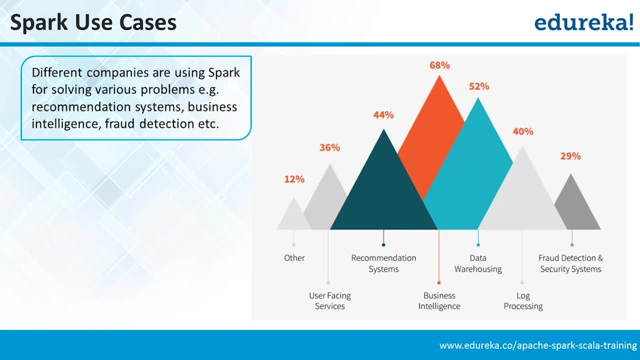 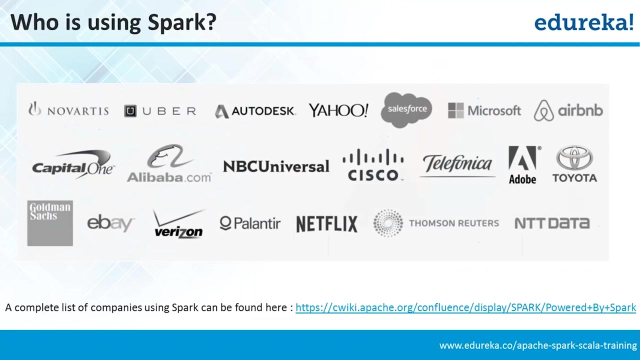 So here are the adoption rate across different techno domain aspects. So, like others, recommendation systems, data warehousing as a data warehousing tool, BI tool, log processing, fraud detection and then user facing service. So this is just like a static slide so you guys can go through any point in time. 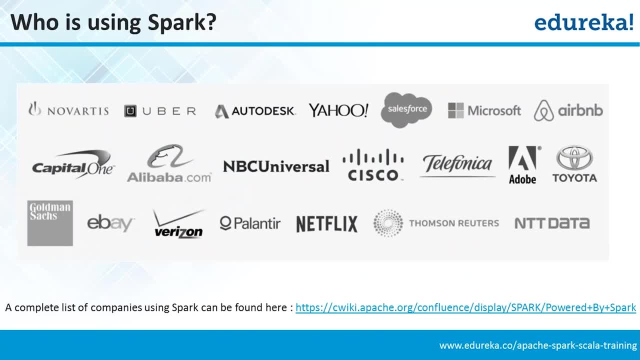 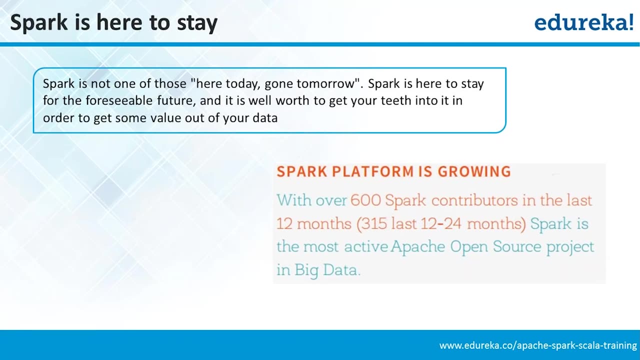 Who is using Spark. So here is the top list of Spark users. Don't worry, these are not the only users. there are plenty of them who have already been adopted to Spark, or at least trying to adopt to Spark. So Spark is here to stay for quite a long time. so now the future is coming for Spark. 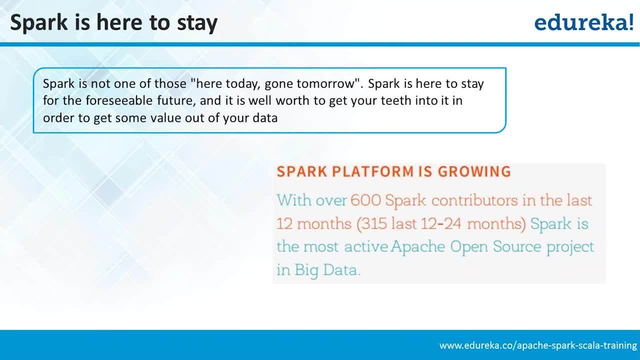 The future is awaiting for Spark, So Spark is not one of those here today gone tomorrow. Spark is here to stay for a significant amount of time and it is well worth to get your teeth into it in order to get some value out of your data. 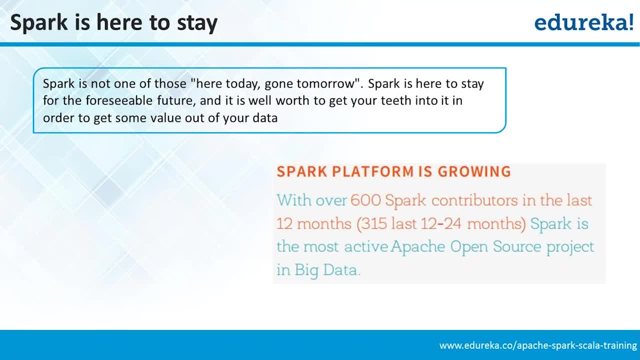 So this is, in fact, this statement is very. I would actually 100% agree with the statement because, with my experience, I personally travel a lot Almost throughout the world. I even travel within the IPAC region quite a number of times. 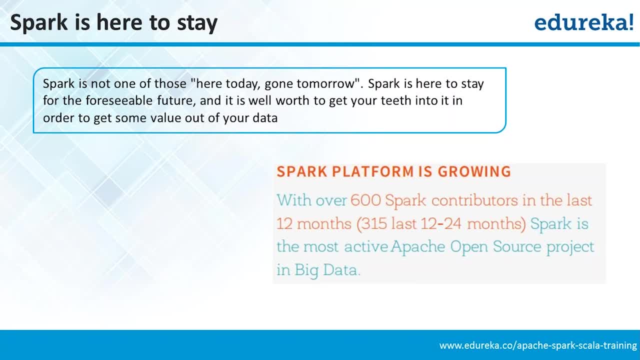 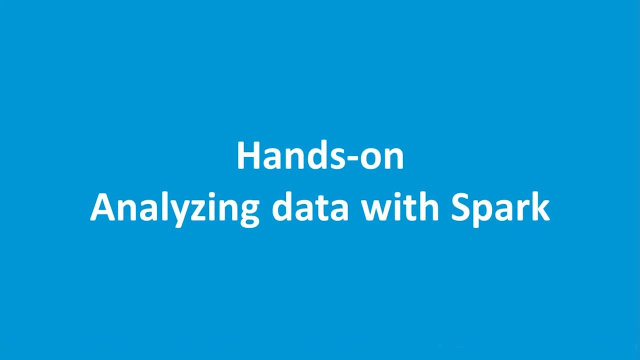 So I personally see many companies are really trying to adopt the Spark framework folks. Okay, so then Spark platform is really growing and here is some information about it. And then let's try to run a quick application. Let's try to run a quick application on top of Spark before we actually wrap up our discussion. 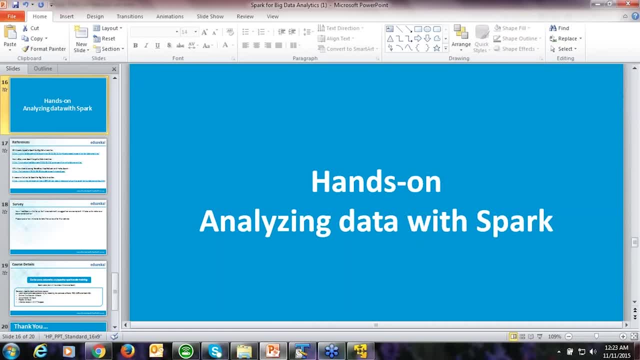 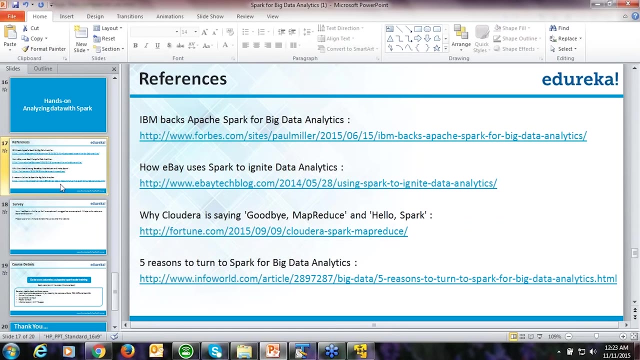 Maybe I'll take just a couple of minutes, not more than that. So, folks, what I'm trying to do basically is okay, so otherwise, I hope that. so this session basically gives you a very good, significant idea on the Spark versus the Hadoop MapReduce. 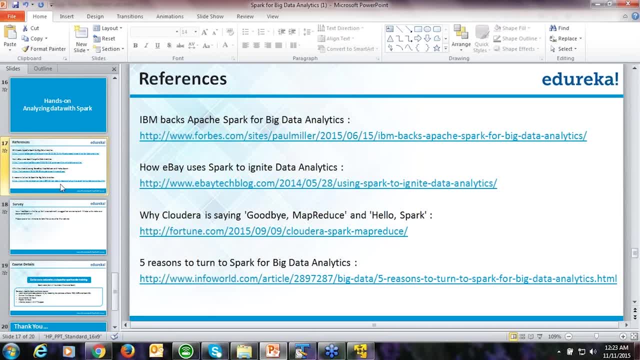 So again, taking another program would be too heavy for us. Okay, so this session basically gives you a very good, significant idea on the Spark versus the Hadoop MapReduce. Once you don't have that wastage of information, you usually can actually go back into stays. 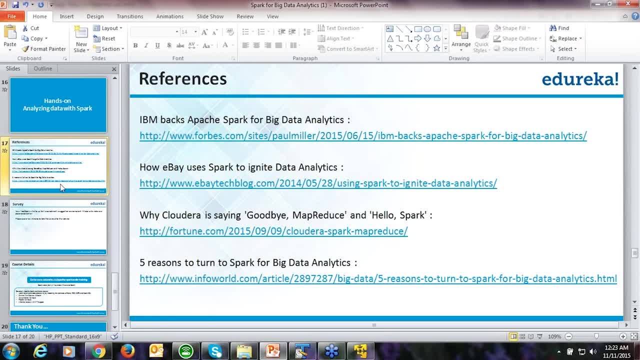 units and into blocks and add additional things if needed. Okay, so this is your first session for today, So I think we've already been able to spend pretty good time in terms of the Hadoop. Okay, so thank you for taking away some of the information. 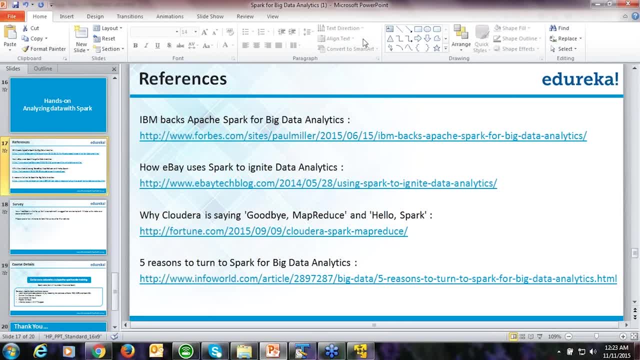 Again, just leave a comment in the Q and A. замечanzzi, or any kind of MATT or what ever ed hemos avido to show and take away from this session. Okay, you can also click today, So you have a lot of information and of course we'll come back to 100 to comment on that. 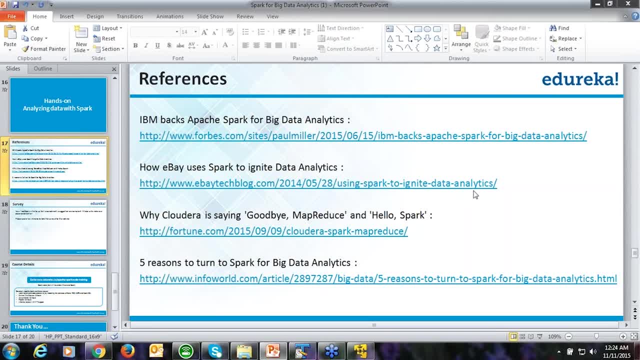 So I have missed few questions which has been posted previously, so please try to post one second. folks, okay, So says prerequisite of experience to go for Hadoop, Linux, Ubuntu, knowledge, programming, knowledge- What is? there is no experience of programming at all. 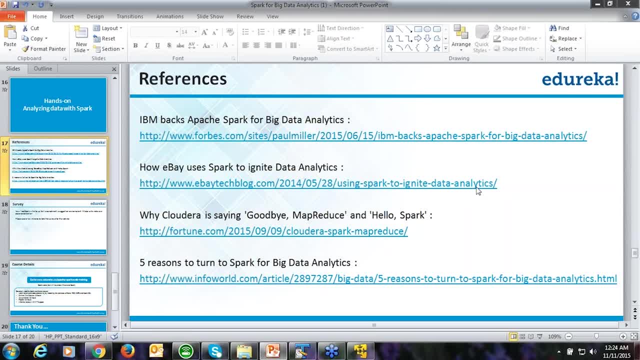 So that's a good question Here. see both- I would say Hadoop and then both. Spark really does not require you to have a very good programming skills, as long as at least you are familiar with SQL skills, And the way the courses has been designed at Edureka is basically to they. let you first 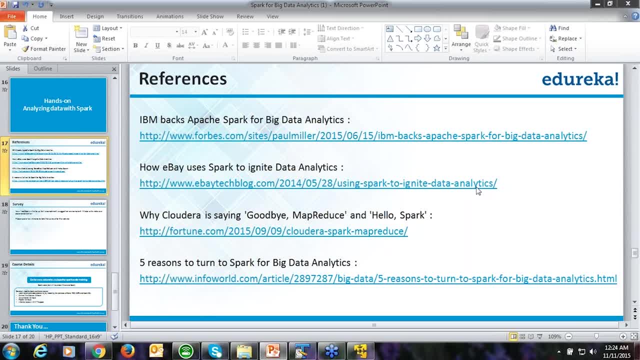 familiar with the programming, and then we'll go on with the programming, Okay, And then we'll go about doing programming. And then there are plenty of other modules, like, if you're talking about Hadoop, there is PIC and High Framework, which does not require any programming skills. 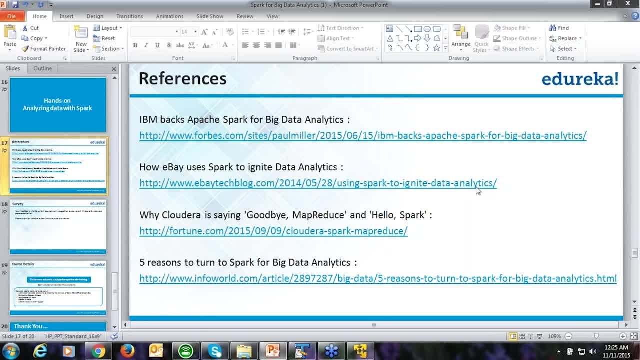 In Spark, for example. Spark SQL does not require any programming knowledge. However, Spark course has been designed in such a way that we'll have very fundamental programming sessions. Maybe for first, two to three sessions will be dedicated for programming Okay, And then we'll get into the programming concepts, where we'll be discussing about the basics. 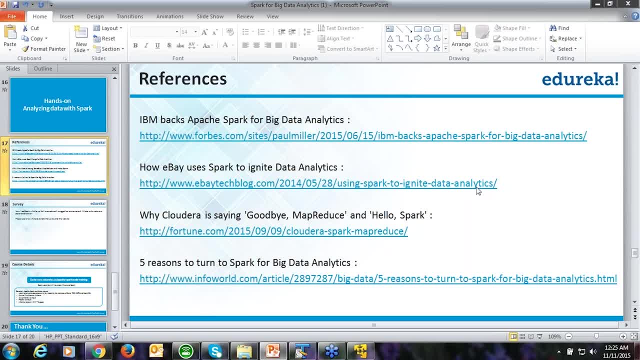 of programming and then we'll get into the actual Sparks discussion, which allows you to quickly adapt to Spark. Pranjal. So I hope your question is too big. I hope in a way I have answered part of it, So I would like to discuss others' questions as well. Pranjal. 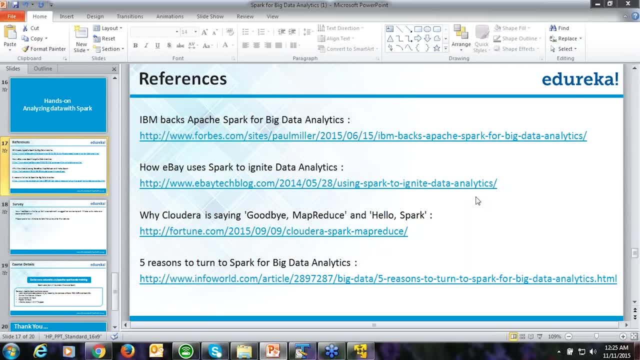 I hope you understand that. So then Karen says: does Spark directly run on data on HDFS or it takes help of MapReduce? Now it directly runs the data on HDFS. It has got its own MapReduce, Kiran. okay. 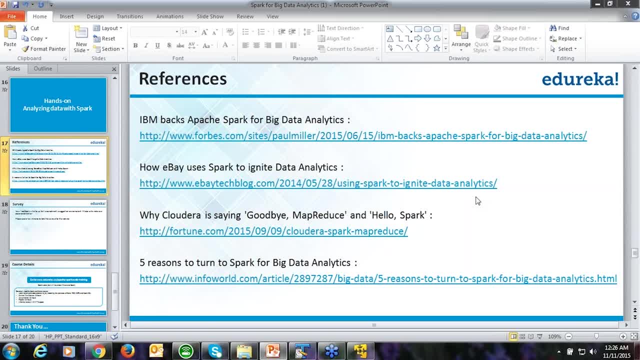 It does not leverage on Hadoop's MapReduce. instead, it uses its own MapReduce, but it still uses On Framework to run its MapReduce applications. okay, Does that answer your question? Samuels says: since Hadoop is developed in Java, what about compatibility, comfort between? 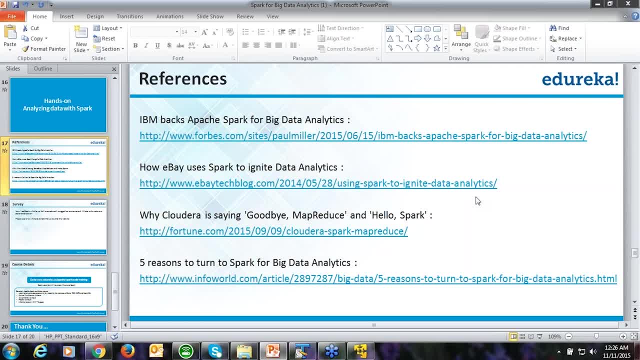 Hadoop and Java. Between MapReduce code and Scala code. Very good question. So Scala and Java- both are like sister languages. okay, So in Scala you could actually use Java code. okay, Most of the APIs in Java can be used directly in Scala, Samuel, which we can discuss in. 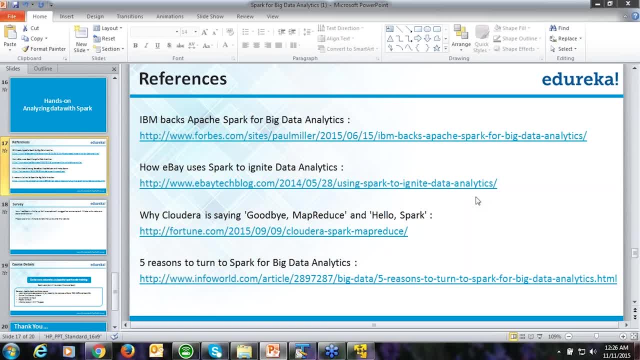 the session. okay, Then what are the prerequisites to learn Spark? Is development background necessary? I hope I have already answered this question to Pranjal. I hope in a way that answers your question too. So it's not mandatory to have pre-programming language as a prerequisite. however, the course 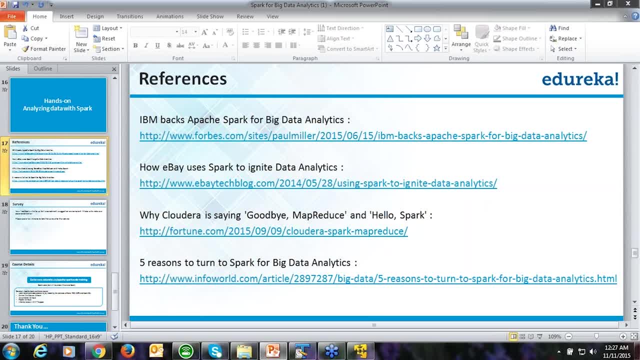 itself will help you to get familiar with the programming and then we'll do the programming in Spark. And also we have got certain models which does not at all require any programming experience. Okay, So Chandra says, Swaroop says: how is Spark different from Hadoop? how is Spark different? 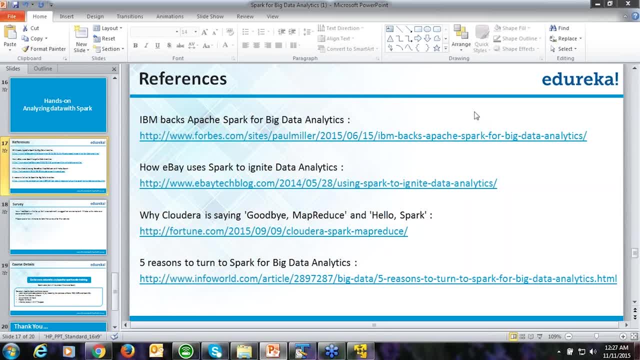 from. Okay, so I hope I have already answered that question, Swaroop. So Hadoop is basically. its core capability is on HDFS Hadoop Distributed File System and it also has got MapReduce, but Spark being the compute engine, you just instead. 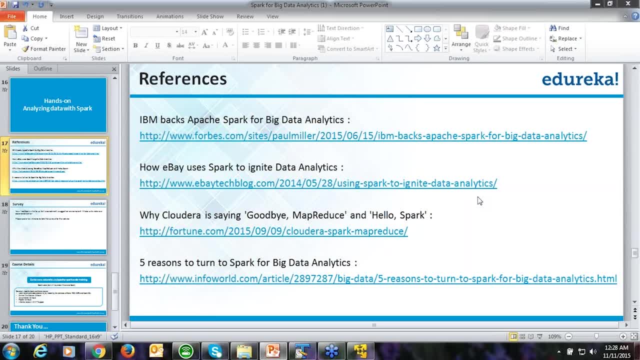 of using Hadoop's MapReduce, You will now leverage on Spark's MapReduce And in Hadoop for doing other type of applications. you have to leverage on other applications, other frameworks. For example, for streaming you have to go with Storm. 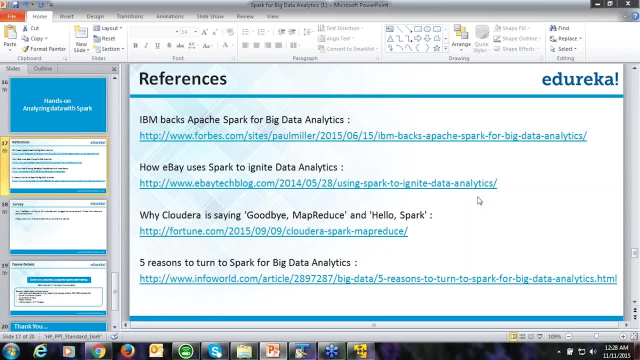 For instance, for graph processing you have to go with Giraffe. So different, different frameworks you have to learn and implement on top of Hadoop. But in Spark everything is packaged as a single framework, so there is very less learning curve. 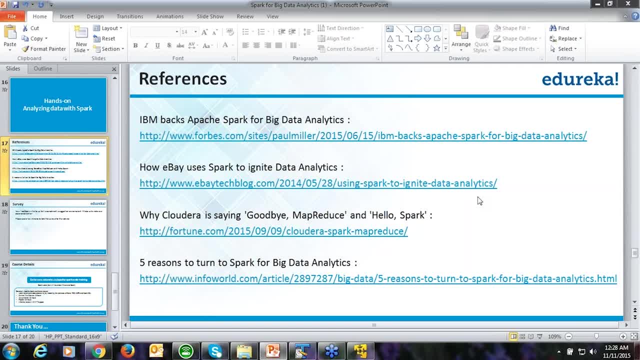 Hope does not. I hope that answered your question. So then, Satya Narayana says I am new learner of Spark. please suggest books. So books, yeah, I mean probably I can request the support team to share the book's links. 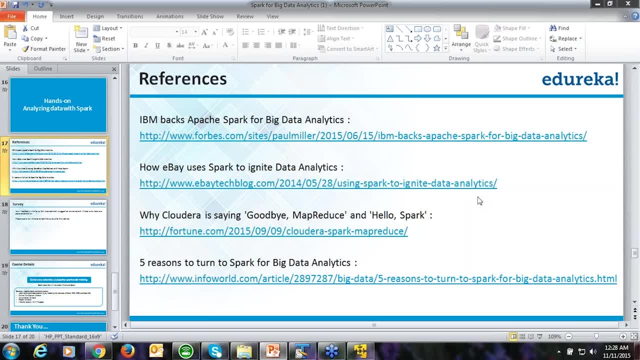 to you, Satya Narayana. okay, Mohan says is Spark similar to SAP HANA in memory technology. So they are not really similar as such, at least in my point of view. I mean, I'm not very, quite familiar with the SAP HANA implementation. 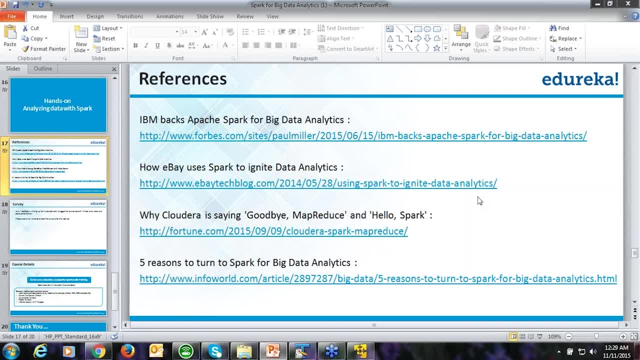 I know how it works, but I'm not quite familiar with that underlying implementation details. However, that's a commercial tool, and then Spark is an open source technology available for us today. Mohan, Then Anand says: are you going to take this Park session? 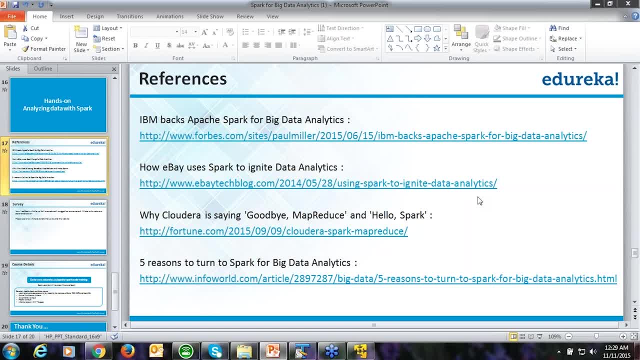 Yes, absolutely Myself, and there are a couple of. There are a few other faculties as well, Anand, Okay, if you are interested in mine, so probably you can actually request the support team. They could be able to assist you when I'm going to start the session, okay. 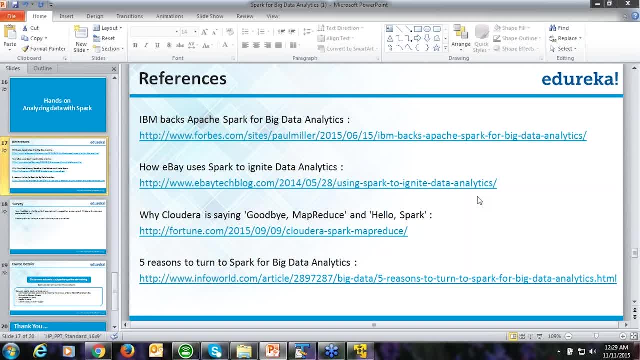 I hope you enjoyed today's discussion as well. Then Vinod says: can I try Spark on MySQL in Windows platform? You can try that, absolutely, Vinod. Then Raghavendra says: is Hadoop course a prerequisite? Yes, absolutely. 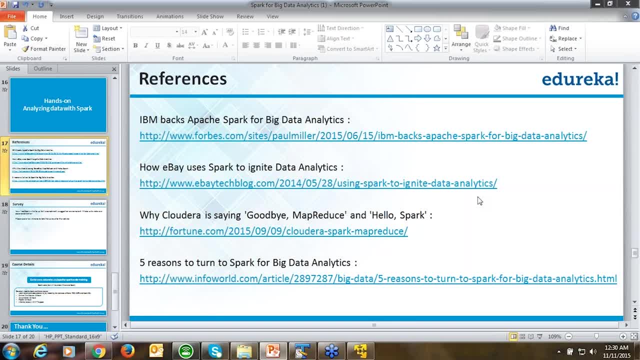 Anand says, is Hadoop course a prerequisite for Spark? Not really. It's not really required to learn Hadoop before you learn Spark. They're standalone In essence. in this course, I'll give you, in fact, some basics of Hadoop as well, which. 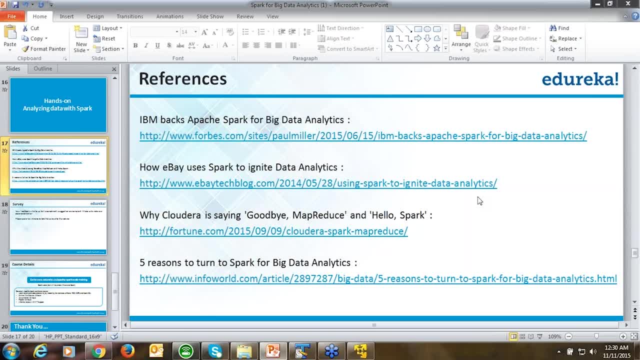 actually help you to distinguish between Hadoop and Spark. Then Anand says okay, then no. So I have already answered that. Anand says I have 10 years of experience in Hadoop. Can I try Spark on MySQL? Yes, absolutely. 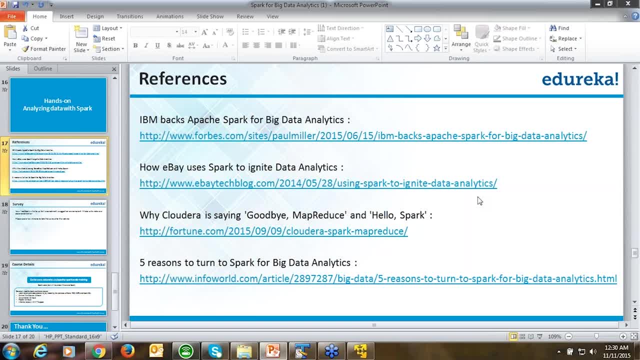 You can try Spark on MySQL. Yes, absolutely, You can try Spark on MySQL. Yes, absolutely, You can try Spark on MySQL. Yes, absolutely. Can I try Spark on MySQL? Yes, absolutely, You can try Spark on MySQL. 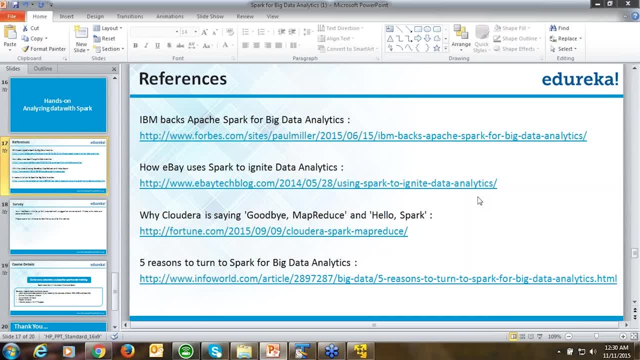 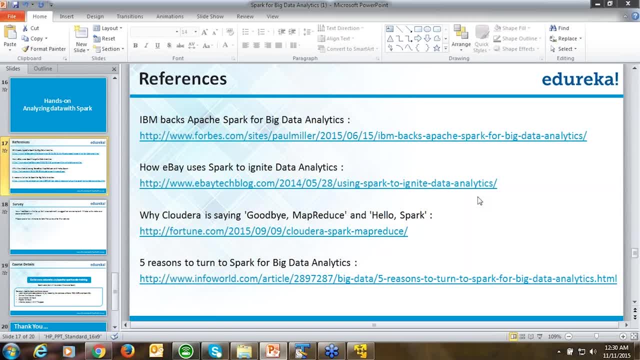 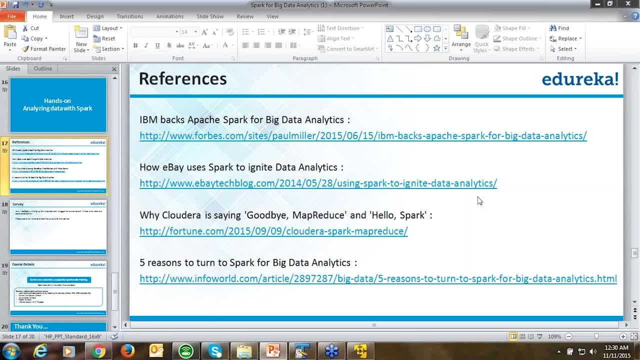 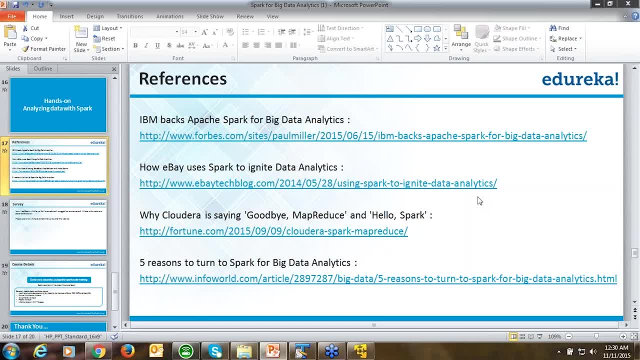 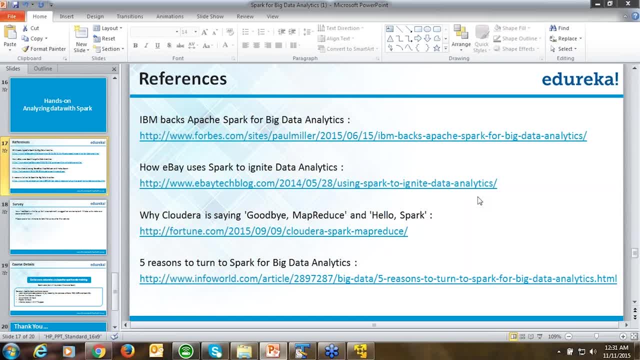 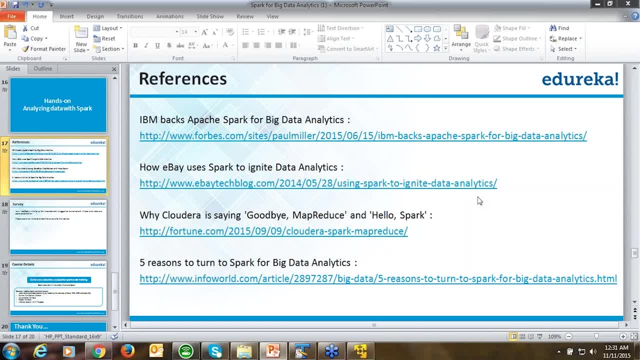 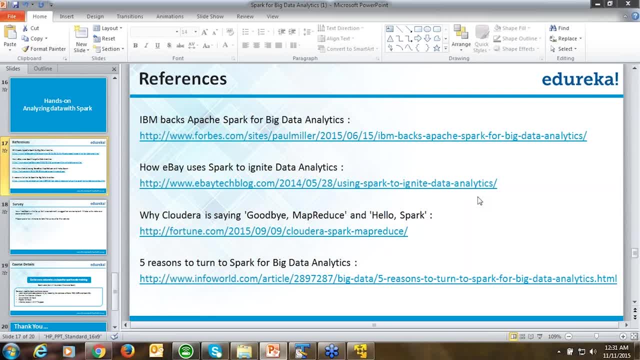 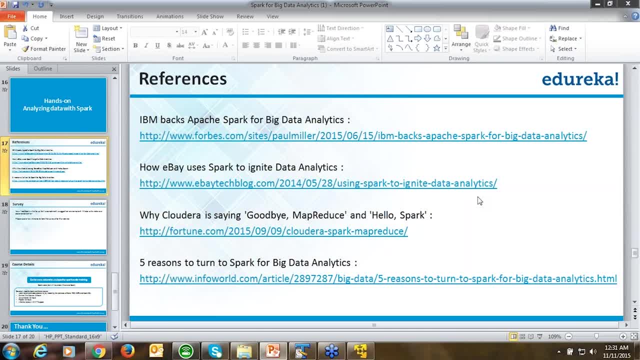 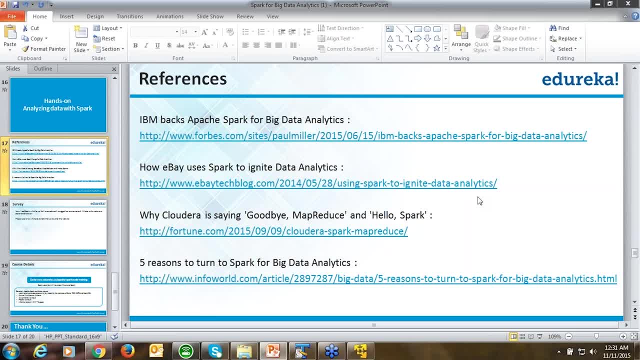 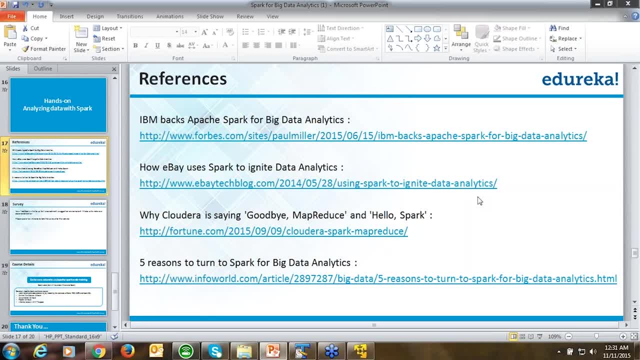 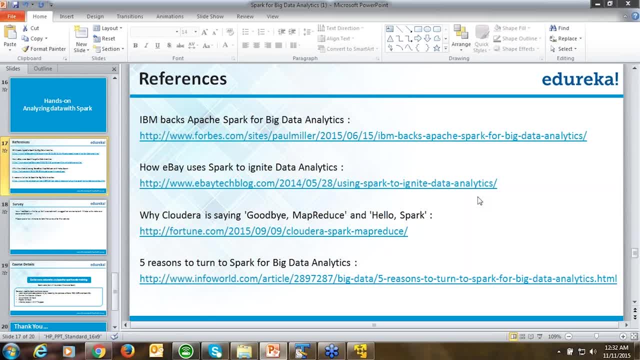 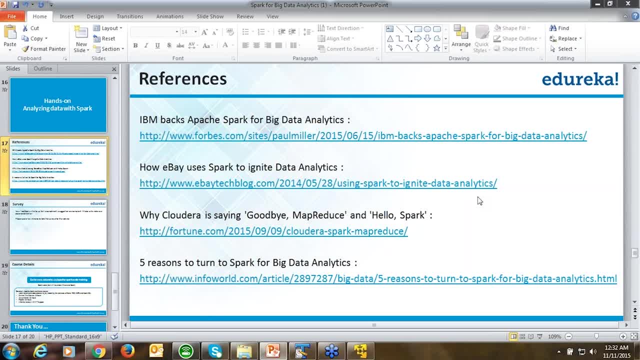 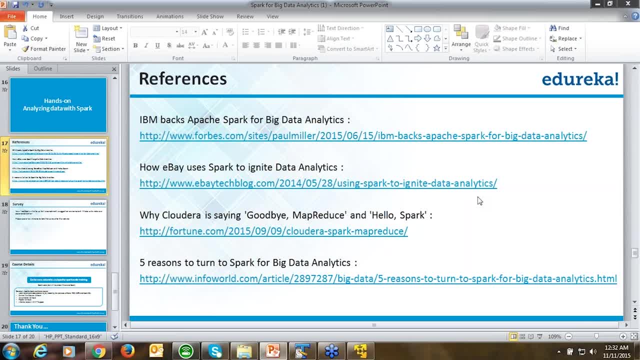 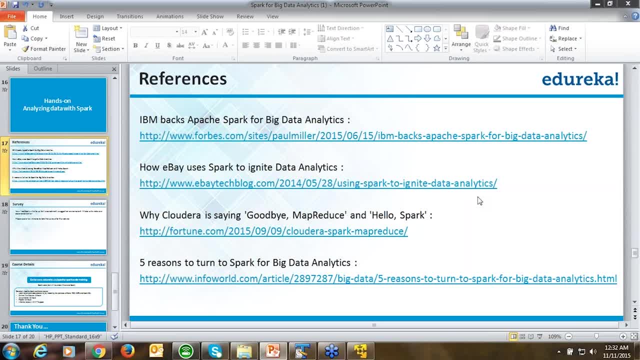 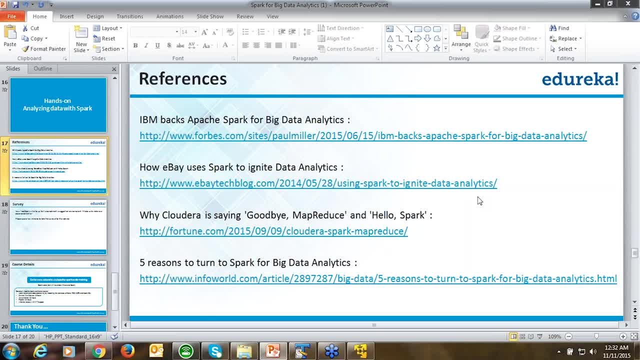 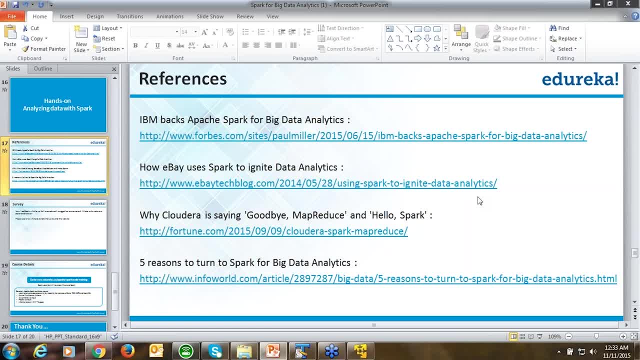 Yes, absolutely, You can try Spark on MySQL. Yes, absolutely, let's try searching for jobs, maybe starting immediately. So, who knows, maybe you can get into your role, maybe within December also. So certain times, I mean, it is quite possible. 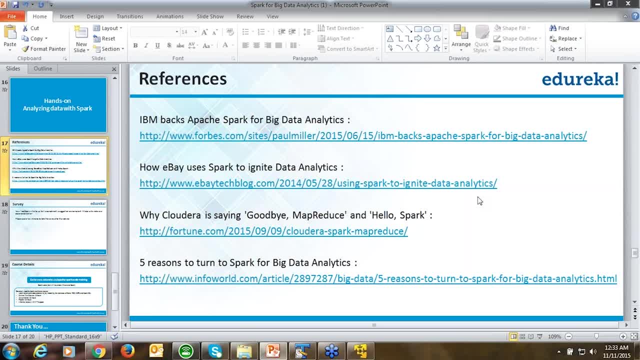 that people could recruit even in December. So again coming back to the other question, since you are not from a Java background, See, Ravi, I had to actually write code in C hash, Maybe like last two weeks back, coincidentally. 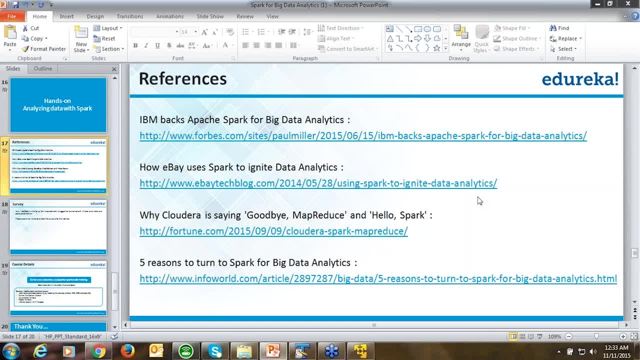 So I'm from Java background. like since my day one, or even before my career has actually started, I did not see much difference between C hash and Java. It's true that it's quite similar, At least vaguely. I can answer that that both of them looks alike to me. 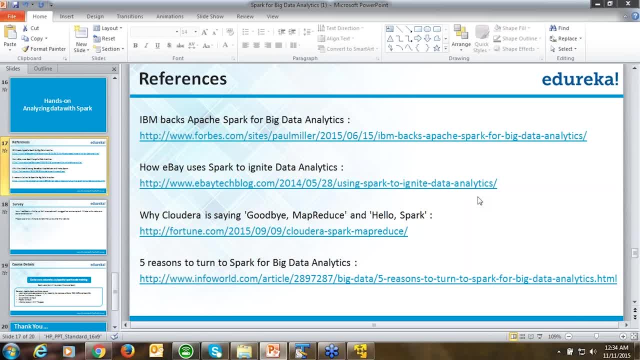 And even when I write applications in other languages, Even write programs in Python. I feel like, as long as you're comfortable in logical thinking, language is just immaterial for you. You just have to understand the syntax. that's it. But again coming back to your specific question, 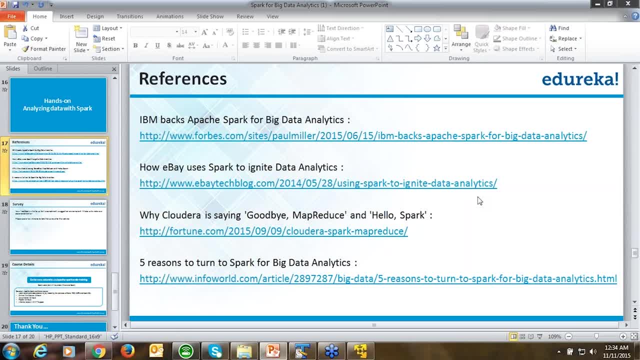 C hash in Java looks pretty much alike and I don't find difficulties in adopting to these two technologies. so I'm sure that you would be able to quickly learn Java if you're from CH development background, and, on the other hand, Scala versus Java. so since you are already learning Hadoop, just continue. 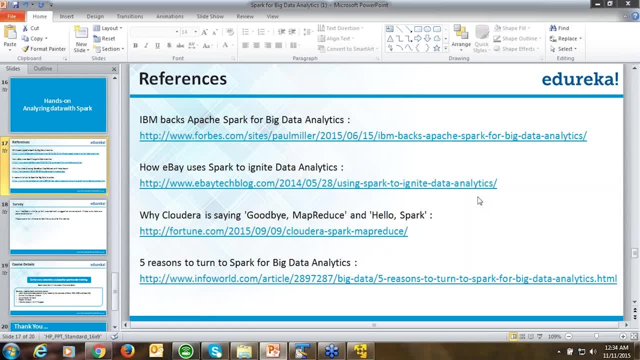 with Java. just get some hands-on experience in Java. if you come for Spark, it is my responsibility to make you familiar with the Scala. Okay, Ravi, does that answer the questions. Then Piyush says: okay, so I want to start my career in analytics. I'm new in this industry, so please. 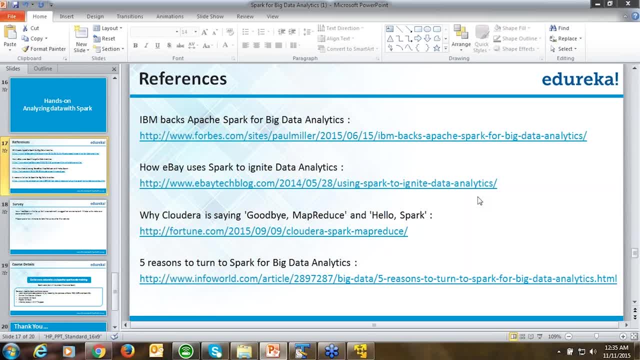 suggest me: shall I proceed learning R language or analytics, or shall I start learning Scala? Okay, so analytics. so what do you mean by analytics? so there are different aspects to it. if you are talking in terms of SQL based analytics, so you can actually go with Spark SQL, and if you are good with 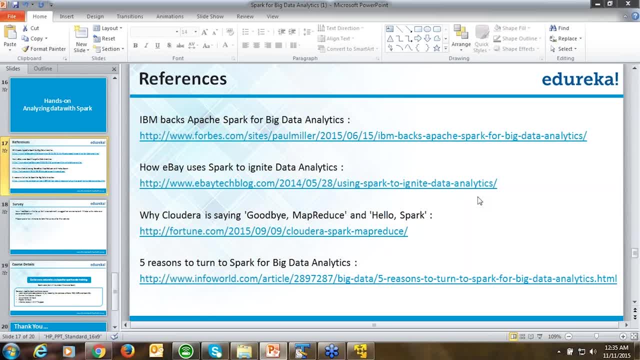 SQL background, then that's fine. If you want to do SQL based analytics, then that's fine. If you want to do SQL based analytics, then that's fine. If you want to do most complex, like complex analytics via mathematical modeling and all statistical analysis, then S you have to learn Scala if at all you want to. 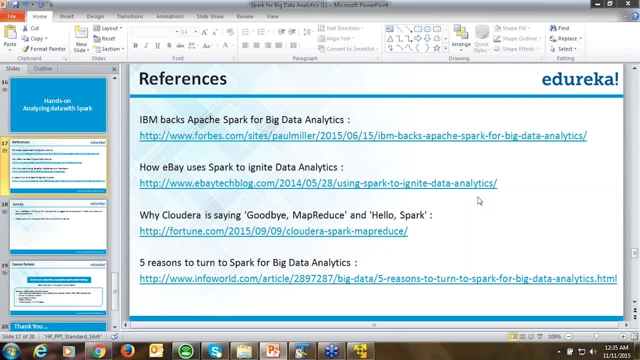 leverage on Spark. So Spark has got MLA package which allows you to run most complex algorithms. so there are plenty of algorithms around there which are, I mean, the most popular algorithms are already available in Spark, so which you could be able to quickly learn. it's not a big deal. and then R is. R is like I. 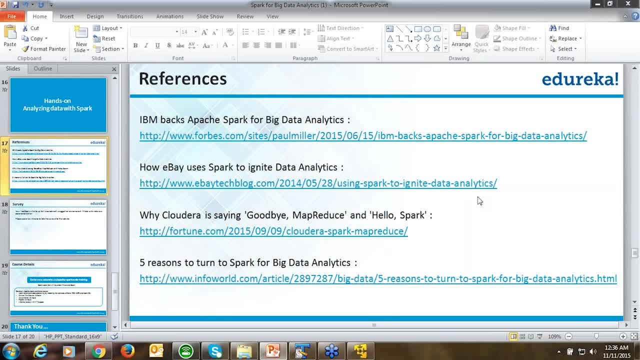 don't want to really compare R with any other language, because R is one of my favorite static statistical tools and the maturity of R is quite, quite higher than any other open source technology, at least in my perspective, in big data domain. So R is a different story altogether, see, if you really want to become a 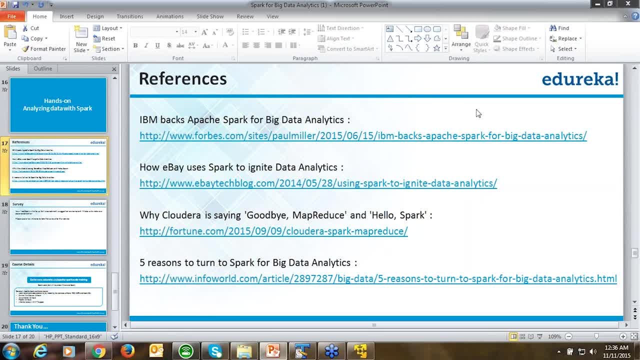 mathematician, I would suggest you to go continue with R and then learn Spark as well. if you are interested in running models and large data sets, okay, and then Shabrish says which programming language would be used in the session. Scala, Shabrish, And Scala is a more prominent language for implementing Spark code. 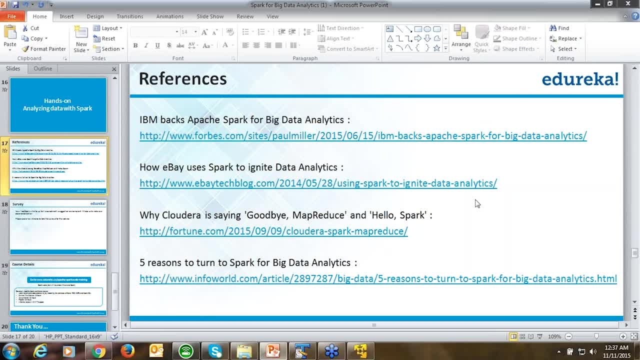 Okay, so I think we're already out of time. maybe I'll take a couple of questions. so my apologies if I couldn't take others questions. I hope you guys understand because of the limited time we have got. and then there are. there were around like 66 folks on the call, so I hope you understand that Samuels is due by the end of the session.